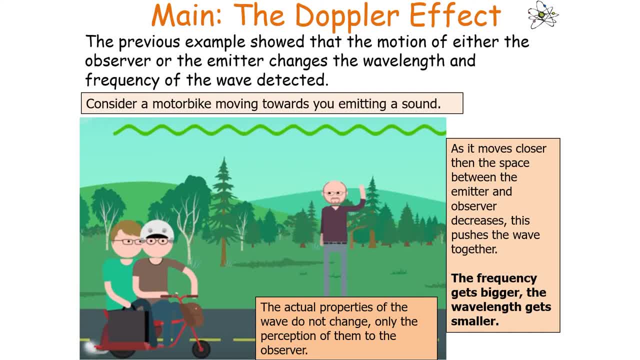 on a motorbike. Now, as the space between the emitter and observer decreases, it will push any wave into the observer. So the Doppler effect is an observational effect as it only changes. the frequency of the wave detected means that the wave emitted closer than the observer. so the 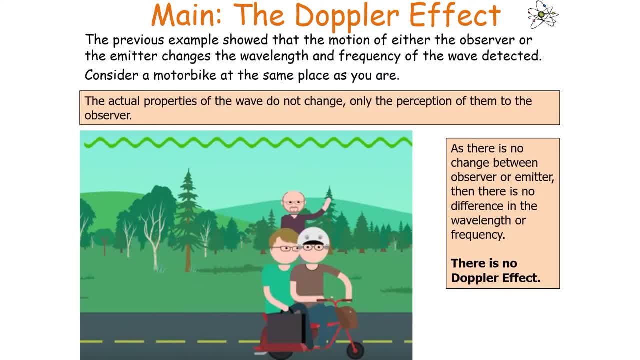 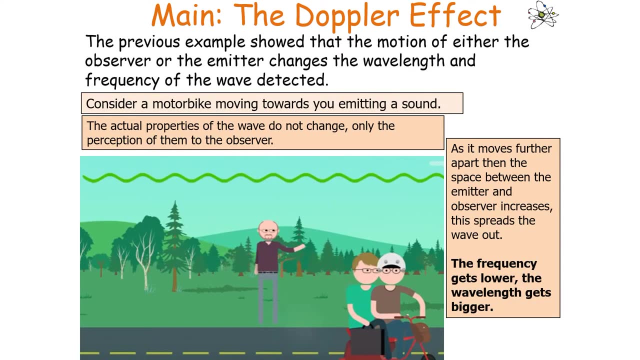 frequency of the wave gets bigger. If the two objects have no change in wavelength and frequency, there is no Doppler effect, And if the emitter and observer moves away from any other focus, the space between the emitter and observer increases, which spreads the wave out. 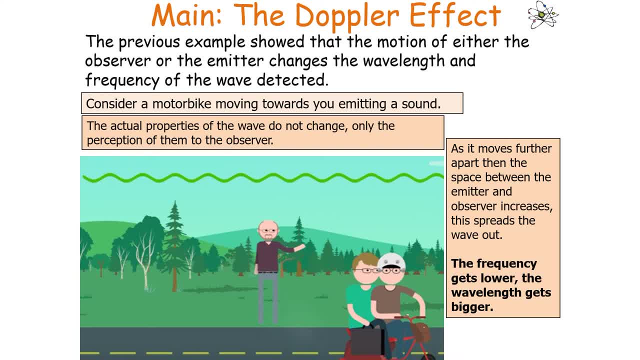 So the E Rec duplicates with that in this scenario and uses the force from the emitter to increase the transmission gets lower and the wavelength gets bigger. This is the Doppler effect. So the Doppler effect is when the wavelength and frequency of a wave is altered by 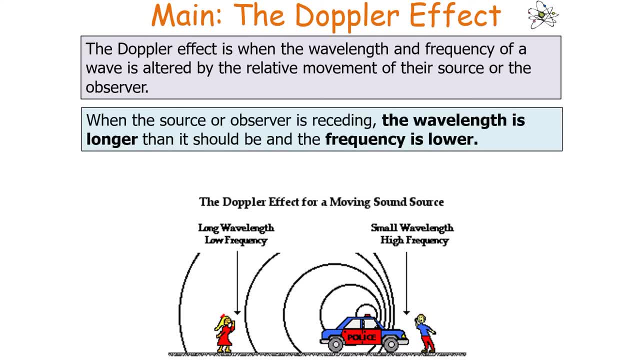 the relative movement of the source or the observer. Now, when the source or observer is receding, moving away from another, the wavelength is longer than it should be and the frequency is lower. Now, when the source or observer is moving towards the other, the wavelength is shorter than it should be and the 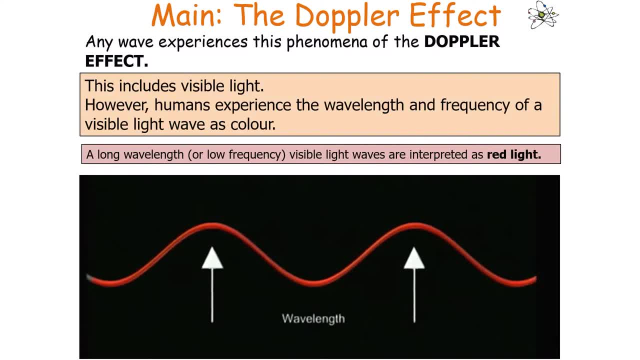 frequency is higher. Now this is important when we consider visible light, because all waves experience the Doppler effect, including visible light, But humans experience the wavelength and frequency of the visible light wave as colour. So what we know is that a long wavelength visible light wave is 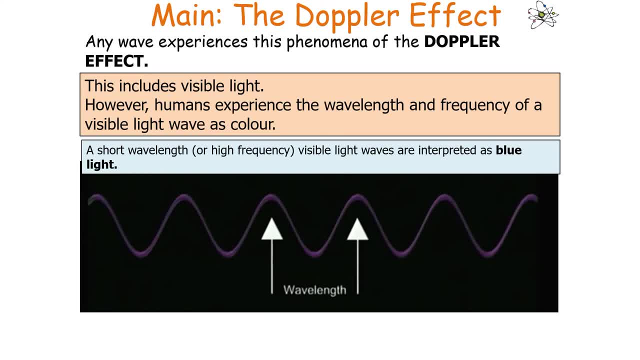 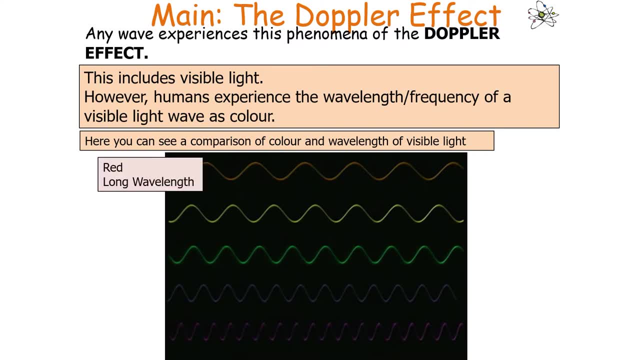 interpreted as red light, whilst a short wavelength visible light wave is interpreted as blue light, which you can see on the following image: here, Our longer wavelength waves are red and our shorter wavelength waves are blue. So now let's consider the Doppler effect from the perspective of 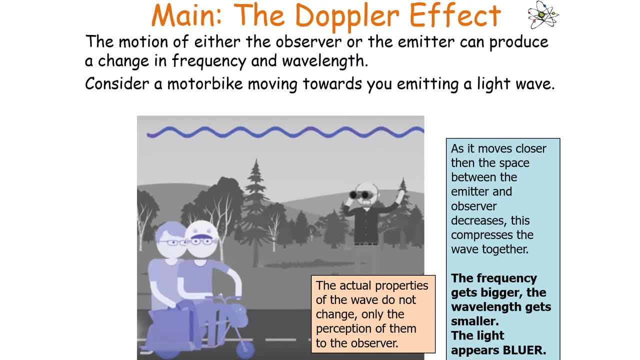 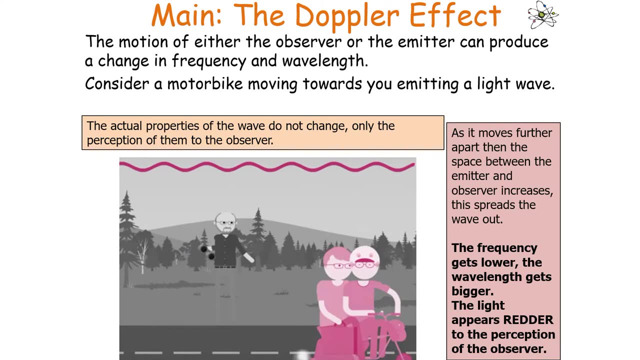 colour, So as the space between an emitter and observer decreases as they're moving towards each other. if there is a light wave emitted, this means that the frequency of the light wave gets bigger. the wavelength gets smaller, so the light appears bluer. Now this is called blue shift. Now, if the two objects 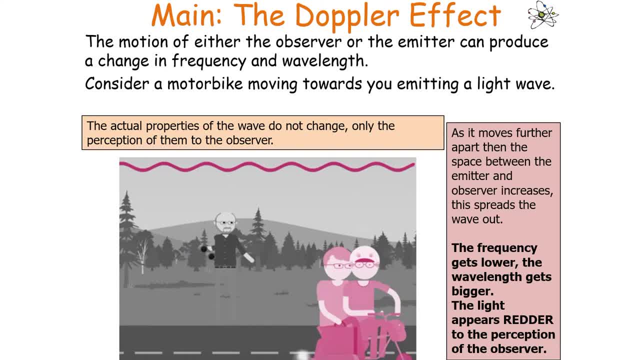 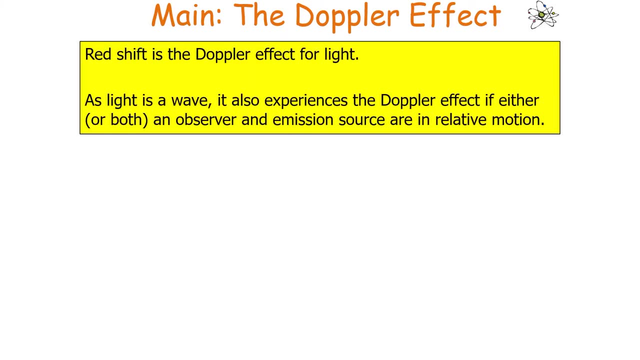 the emitter and the observer are moving further apart. well, the space between the two objects increases, so therefore the frequency gets lower and the wavelength gets bigger. so the light appears redder to the perception of the observer. We call this red shift. So red shift is the 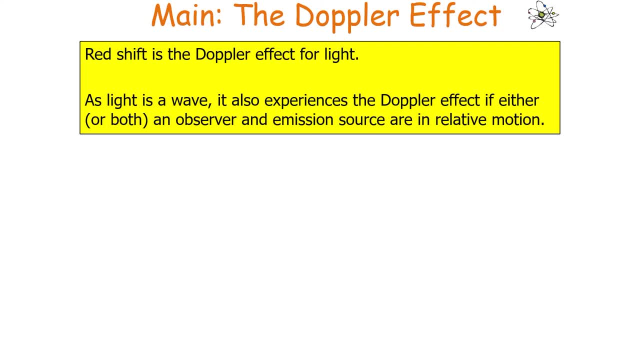 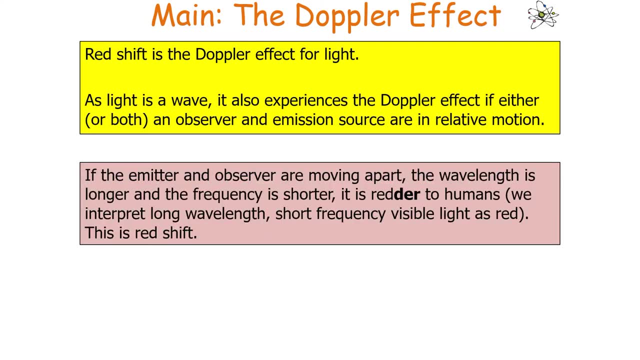 Doppler effect for light. Now, as light is a wave, it experiences the Doppler effect if either or both an observer or an emission source are in relative motion. So if the emitter and observer are moving apart, the wavelength is longer and the frequency is shorter, so it appears redder to humans. This is red shift. If the two 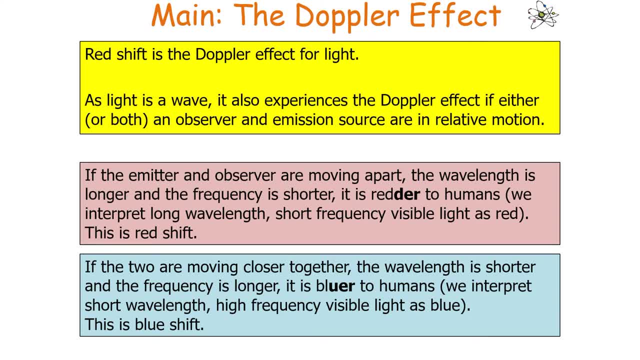 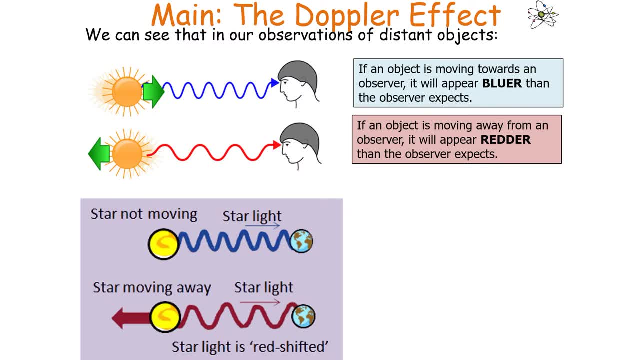 objects are moving closer together, the wavelength is shorter and the frequency is longer, so it appears bluer to humans. This is blue shift, So we can observe this in the example of distant objects in our universe. If an object is moving towards an observer, it will appear bluer than the observer expects. 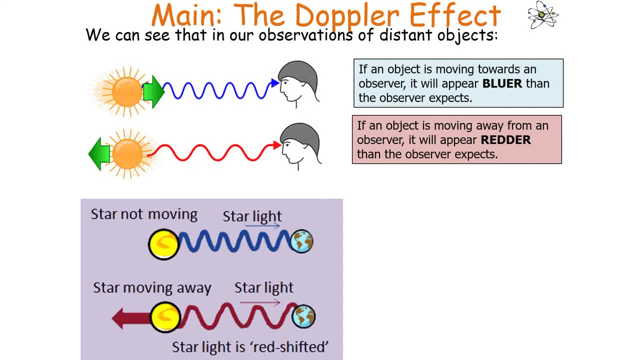 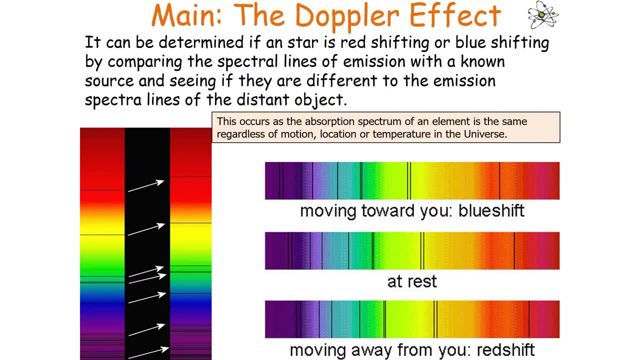 But if an object is moving away from an observer, it will appear redder than the observer expects. Now we can determine if a stellar object is red shifting or blue shifting by comparing the spectral lines of emission with a known source and seeing if there's a difference to the emission spectral lines of that distant object. 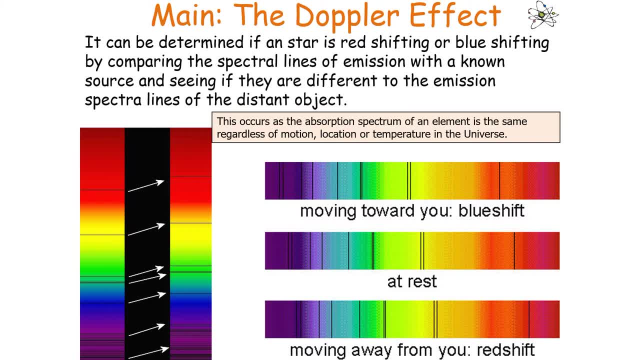 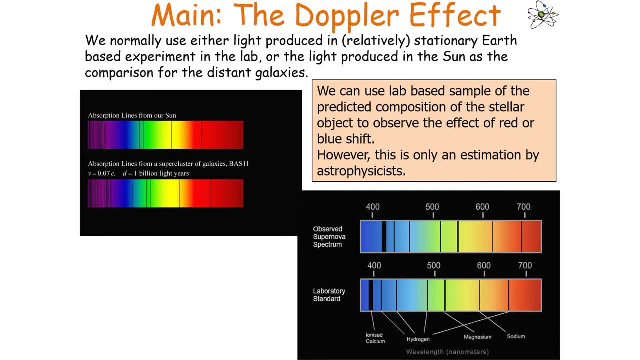 This occurs as the absorption spectrum of an element is the same regardless of motion, location or temperature in the universe. So we can use a lab-based sample of the predicted composition of a stellar object to observe the effect of red shift or blue shift. This 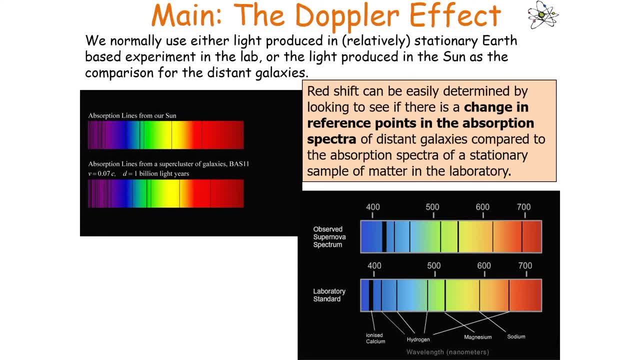 can take place because we can see if there's a change in reference points in the absorption spectrum of distant galaxies. The most commonly used reference points are the Barmer lines, the visible absorption lines of hydrogen, because hydrogen is the most common element in the universe. 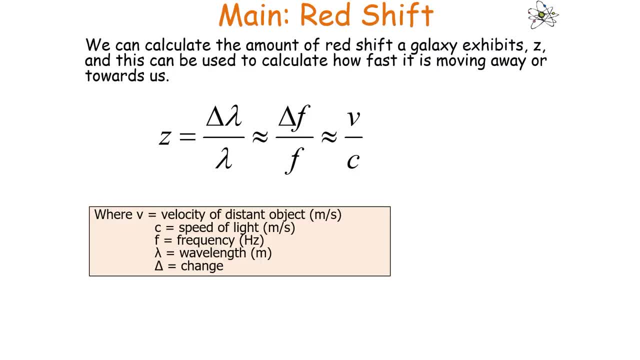 Now we can calculate the amount of red shift. a galaxy exhibits Z with the following equation: Z equals the change in wavelength over wavelength, which equals the change in frequency over frequency, which is equal to the velocity of the moving object. It all comes down to this equation. 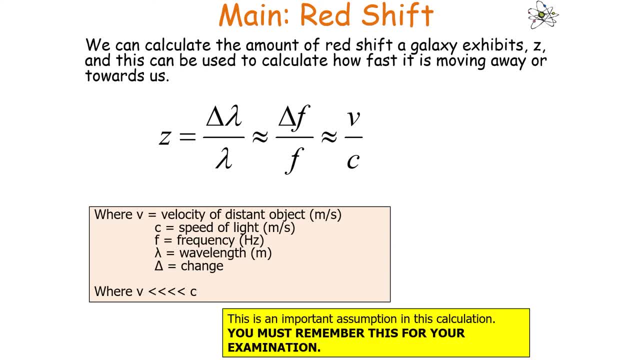 It is important to remember that in this equation, it will only work if the recession velocity is much less than the speed of light, which is a important idea. Now you are given these equations in your examination, but you've got to be able to. 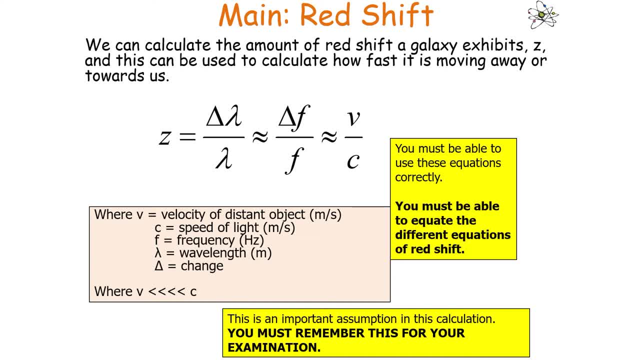 use these equations correctly. So you've got to be able to equate the different equations of redshift. So you can say that a change of wavelength over wavelength equals the speed of light. So you can see here that there's a big difference between speed of light and the speed of light. 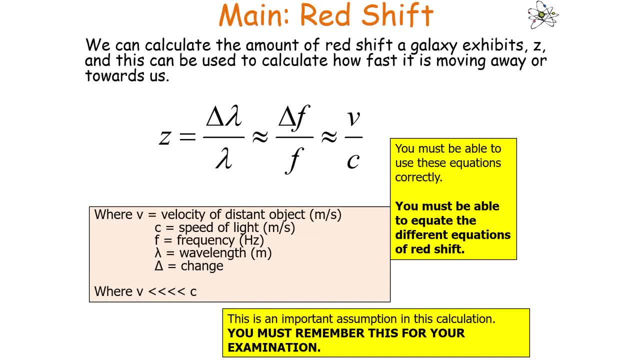 which is just an example of the speed over wavelength over wavelength is equal to the velocity over the speed of light. or you could say: change in frequency over frequency is equal to the change in wavelength over wavelength, or any iteration you would like, but you can equate them to each other. Now, Z is a quantitative measure of the. 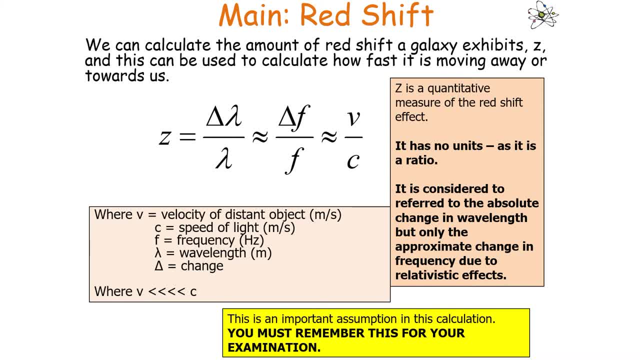 redshift effect and it has no units. It is a ratio. Now it can be considered to be the absolute change in wavelength, but only the approximate change in frequency due to relativistic effects. Now Z is positive if the object is redshifting, but Z is negative if the object is blueshifting. 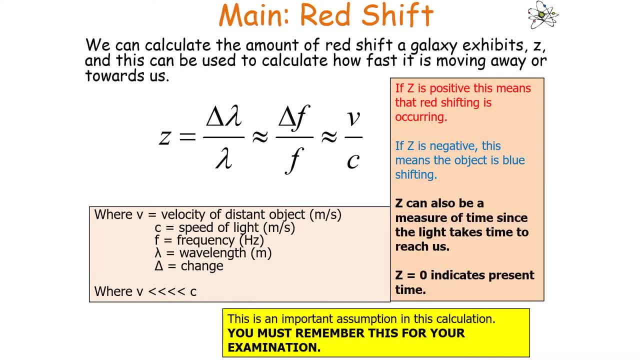 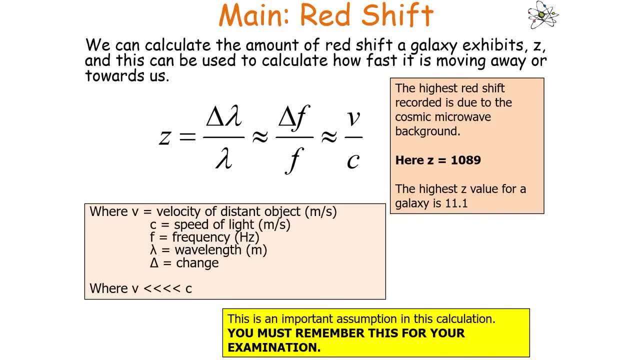 Now, Z can also be a measure of time, since the light takes time to reach us. So if you see the notation, Z equals zero. it indicates the present time. Now. the highest redshift ever recorded was due to the cosmic microwave background radiation, with a redshift of 1,089,, whilst the highest Z 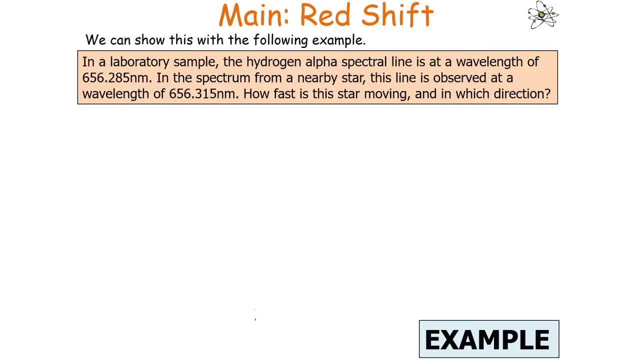 value for a galaxy is 11.1.. Now we can look at carrying out a calculation with the following example. In a lab sample, the hydrogen alpha spectral lines had a wavelength of 656.285 nanometers In the spectrum from a. 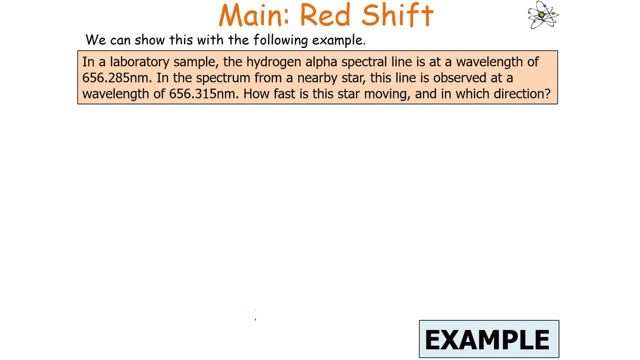 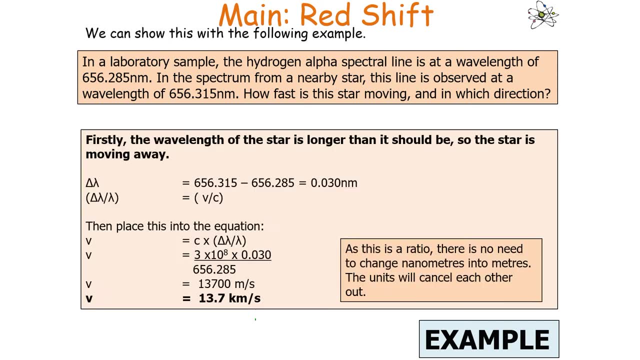 nearby star. this line is observed at a wavelength of 656.315 nanometers. How fast is this star moving, and in what direction? Well, the first thing you can note is that the wavelength of the star is longer than it should be, so it must be moving away Now. the next thing you can do is that you 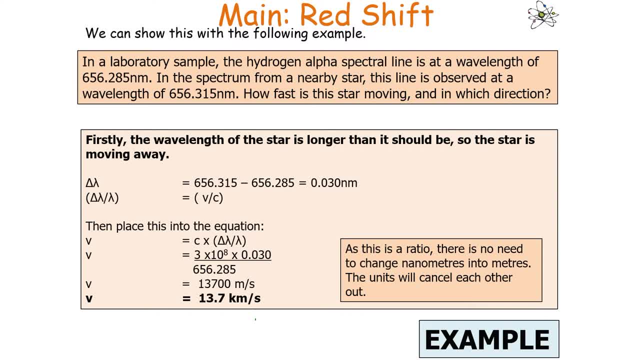 can work out what. the wavelength of the star is longer than it should be, so it must be moving away. V is going to be, by thinking of the equation: change in lambda over lambda is equal to V over C. so therefore, V is equal to C times by change in lambda over lambda. Now, as this is a ratio, 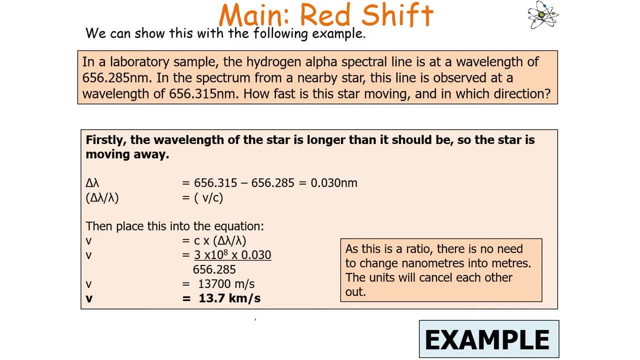 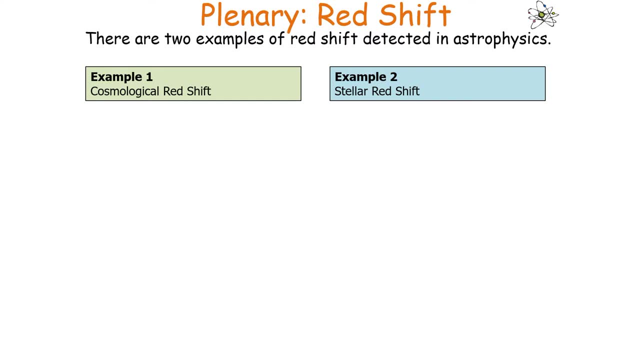 there's no need to change your wavelength from nanometers into meters, because they'll just cancel through each other anyway. So you work your answer out to be 13700 meters per second, or 13.7 kilometers per second. Now there are two examples of redshift detected in astrophysics. There's 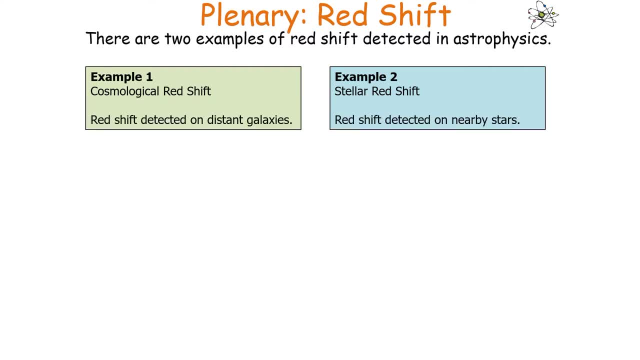 the cosmological redshift, and there's also stellar redshift. The cosmological redshift is redshift detected on distant galaxies, while stellar redshift is redshift detected on nearby stars. Now, cosmological redshift is detected on all galaxies except the Andromeda, whilst stellar redshift is detected on certain stars. 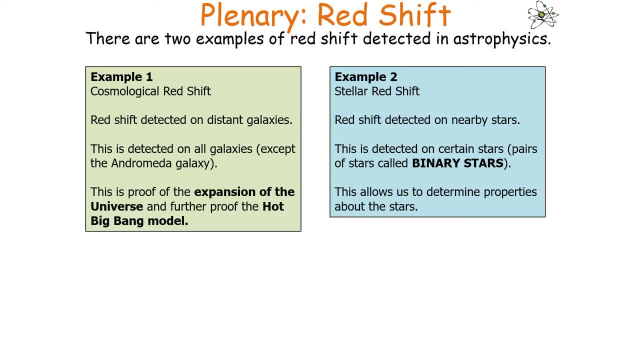 especially pairs of stars called binary stars. Now the cosmological redshift allows us for further proof of the expansion of the universe and the hot big bang model, while stellar redshift is allows us to determine properties about stars. So let's consider stellar redshift. 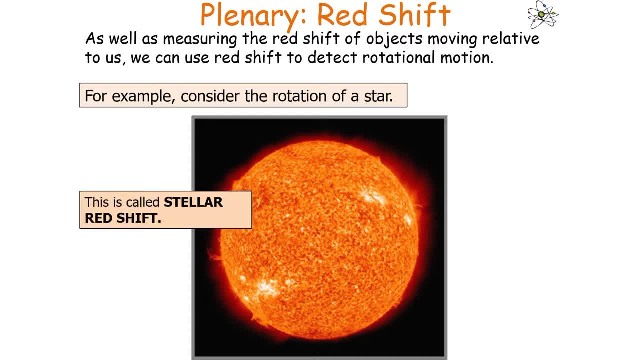 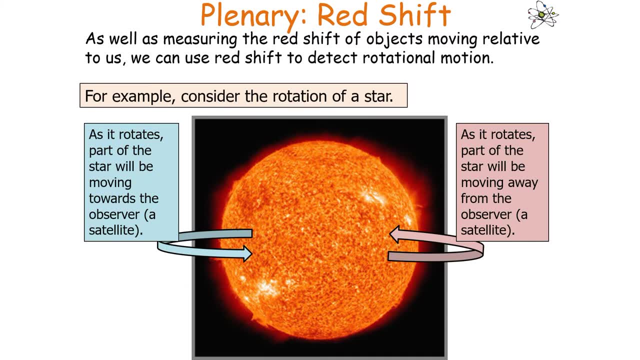 So let's consider the rotation of a star in this concept of stellar redshift. Now we will observe red and blue shift with stars due to their rotational motion. So as the star rotates, the part of the star will be moving towards an observer. 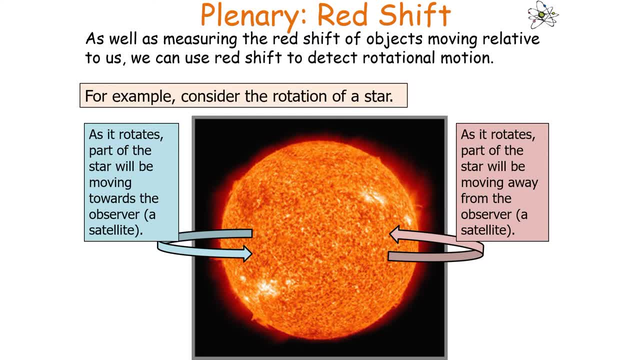 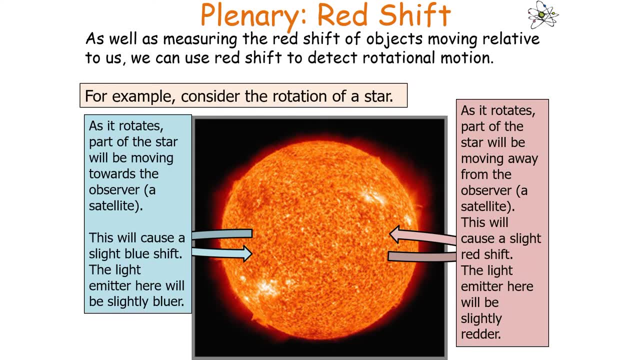 such as a satellite, and as the star rotates, part of the star will be moving away from an observer such as a satellite. So the part of the star moving towards us will produce light which is slightly blue-shifted, So the light emitted from this part of the star will be slightly bluer. 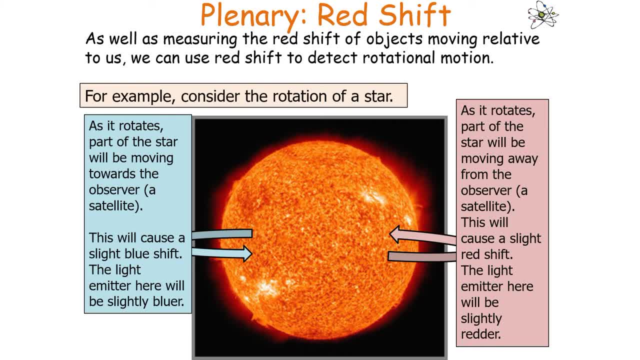 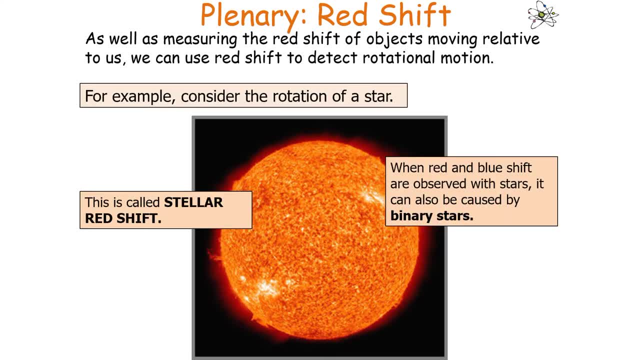 whilst the part of the star rotating away from us will have a slight redshift in the light emitted, which will be slightly redder, which is how we can determine stellar rotation. Now we can also observe this idea of redshift and blue-shift with binary stars. 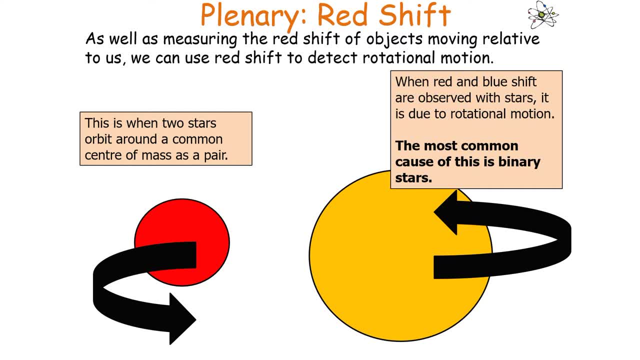 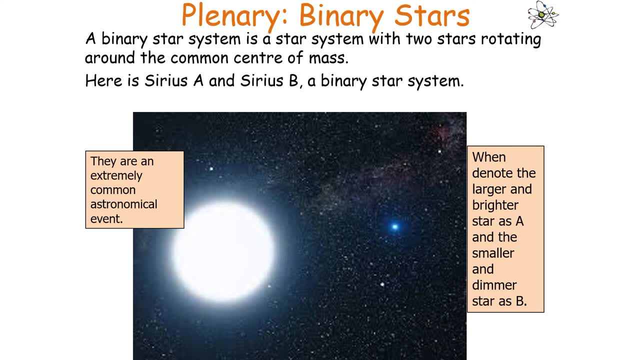 So binary stars are when you have two stars orbiting around a common centre of mass as a pair. Now this is an extremely common astronomical event. Now we tend to denote the larger and brighter of the two stars as the A star and the small and 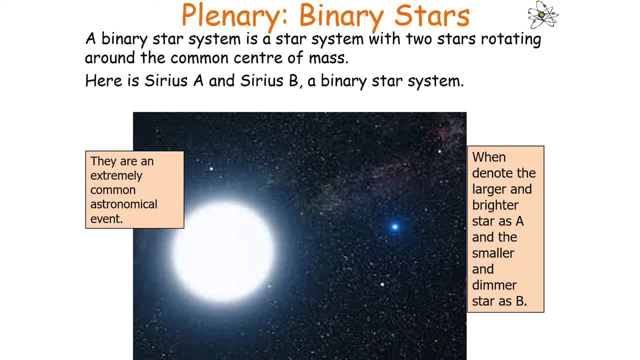 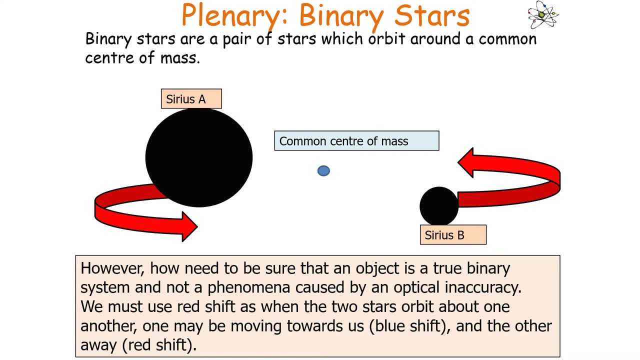 dimmer of the two stars as the B star, So we've got Sirius A and Sirius B as shown in this diagram. Now we need to be sure, though, when we're observing these binary stars from Earth, that these are actually true. 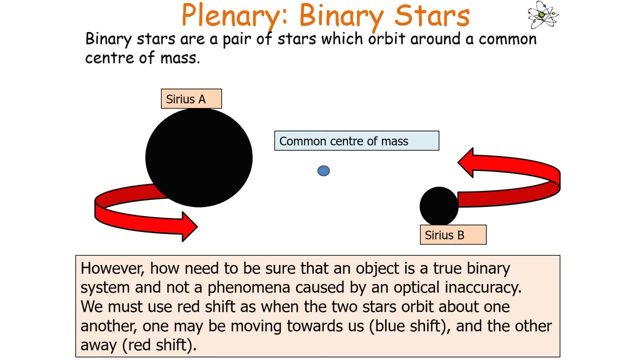 but a binary system and not a phenomena caused by optical inaccuracy. So we've got to use redshift is on the two stars orbiting about one another. One will be orbiting towards us and one will be orbiting away from us. 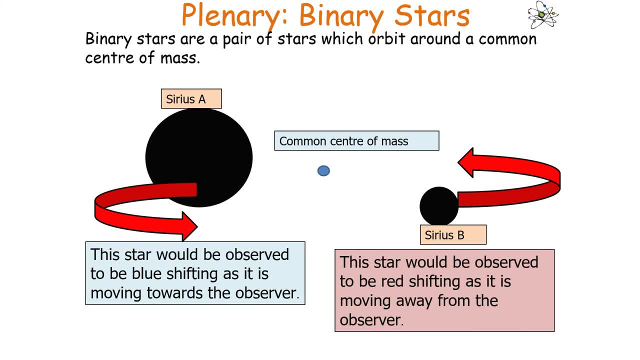 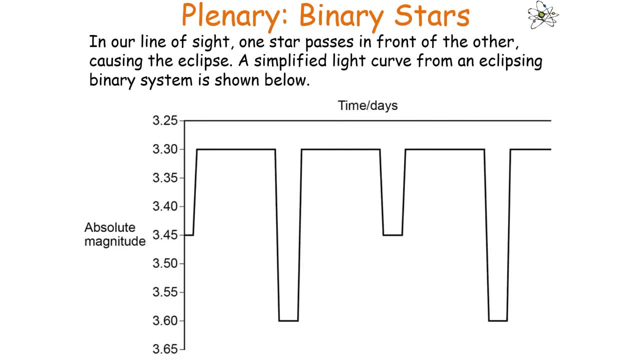 So star which will be moving towards us would blue shift, the light from the star blue shift and the star observed removing away from us would have light emitted which is red shifted. so, in our line of sight, one star will in fact pass in front of the other, causing an eclipse which you can see. 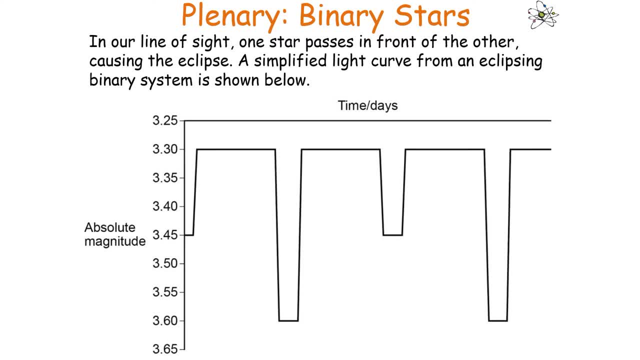 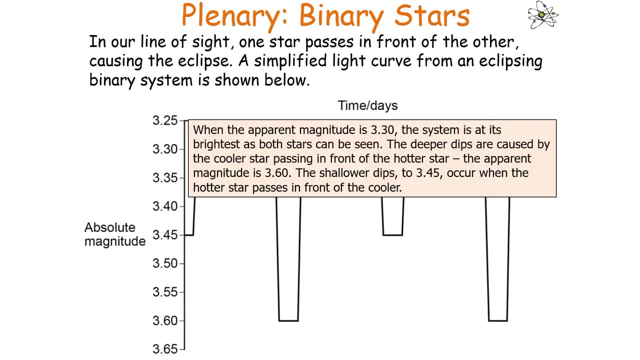 in the simplified light curve for an eclipse and binary system shown below. so the apparent magnitude scale increases going downwards, ie the dips in the graph correspond to the light dimming, and in this example the two stars have different surface temperatures so actually might emit different amounts of light anywhere per unit surface area. so when the apparent magnitude is, 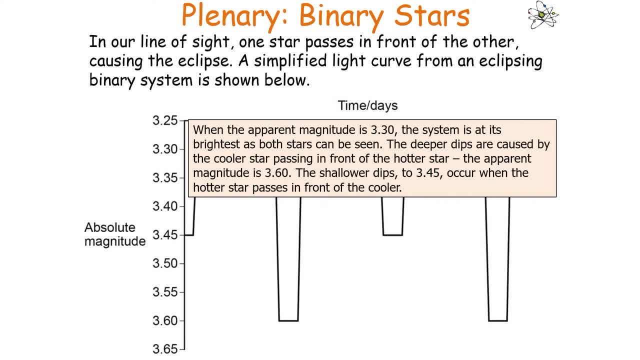 3.30. the system is at its brightest as both stars can be seen from earth. now, the deeper the dips are caused by the cooler star passing in front of the hotter star, or so the apparent magnitude is 3.60. now the shallower dips, that to 3.45, occur on the hottest star passes in front of the cooler. 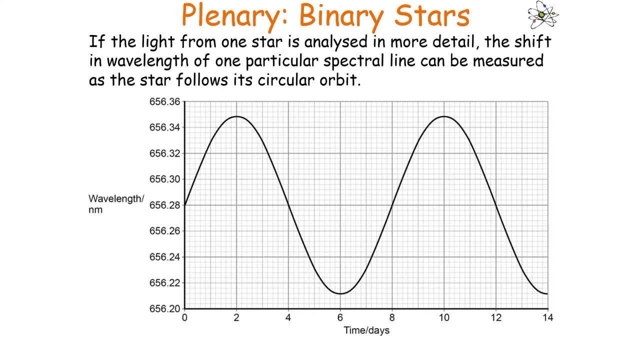 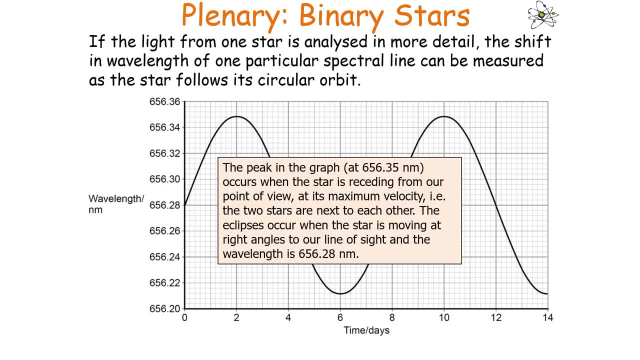 now, if the light from one star is analyzed in more detail, the shift in wavelength of one particular spectral line can be measured as the star is moving towards us. so the difference between the two stars follows its circular orbit. so the peak in the graph occurs when the star is receding from our 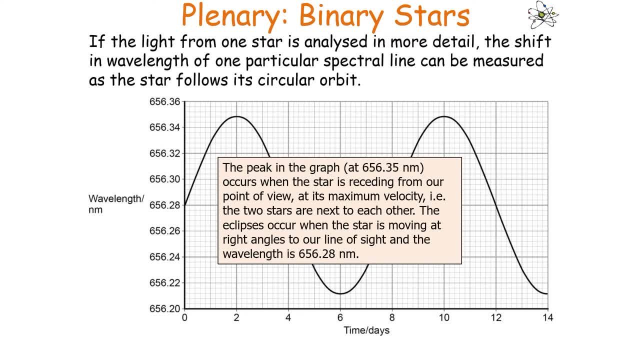 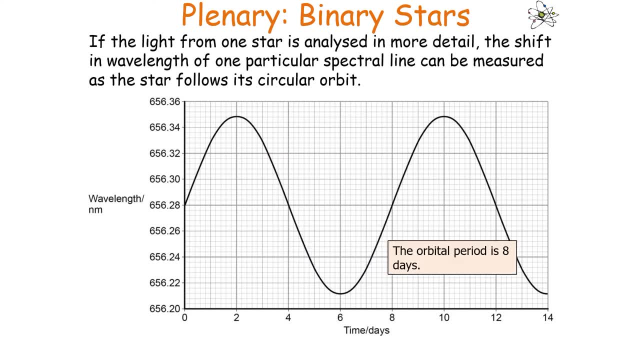 point of view at its maximum velocity, and the eclipse occurs when the star is moving at right angles to our line of sight. so you can see from this particular image that the orbital period will be eight days, as this is how long it takes before the wave repeats itself. you can then use 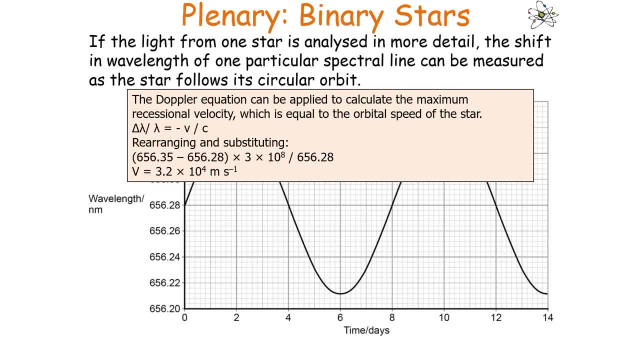 your doppler equation. to calculate the maximum recession velocity, which is equal to the orbital speed of our star, by doing change in lambda over lambda equals v over c. to work out the velocity of our star by doing change in lambda over lambda equals v over c. to work out what v would be: 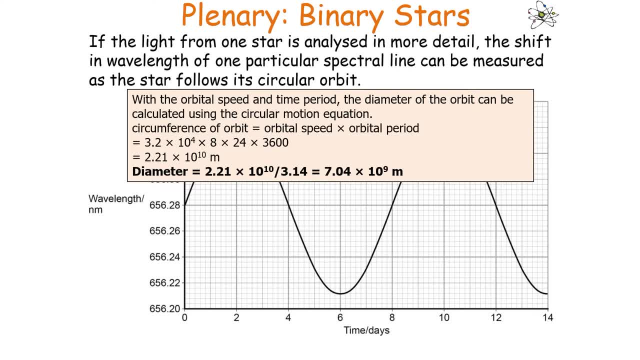 you can then, with the orbital speed and the time period, determine the diameter of the orbit by using a circular motion equation where the circumference of the orbit is equal to the orbital speed times by the orbital period, and so, as a result, you can work out your diameter of your 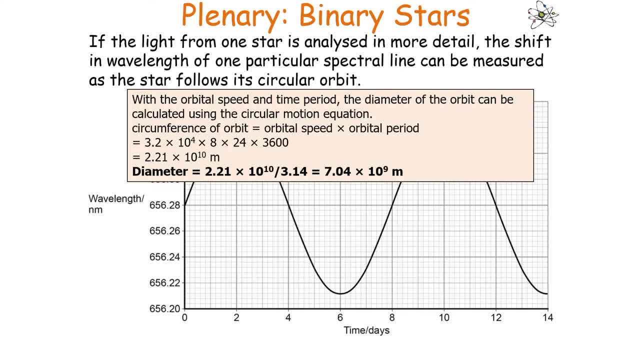 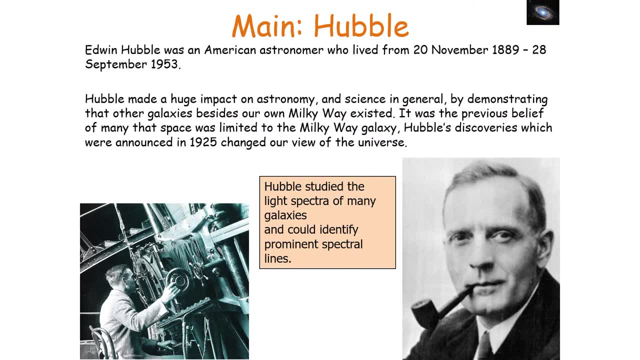 orbit by doing your circumference divided by pi. so now let's look at hubble's law now. edwin hubble was an american astronomer who lived in the early 20th century now. he made a huge impact on his astronomy now. hubble studied the light spectra of many galaxies and could identify prominent 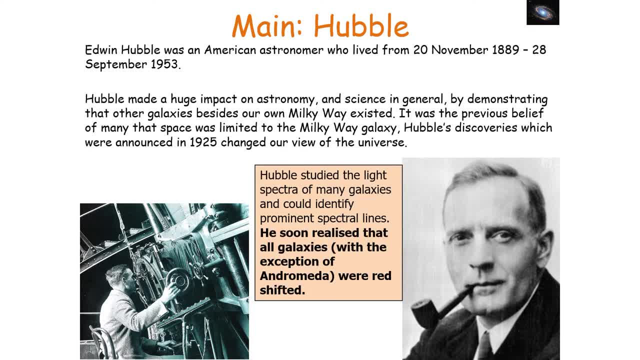 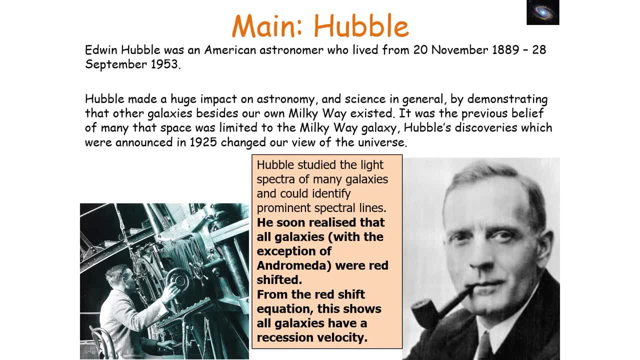 spectral lines. now he soon realized that all galaxies were redshifted. so from the redshift equation it shows that all galaxies were moving away from the earth. so all galaxies have a recession velocity. now hubble deduced the distance from earth that these galaxies have by using 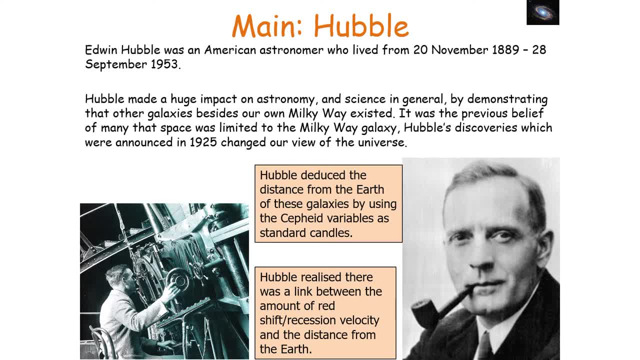 separate variable stars as standard candles. now hubble soon realized there was a link between the amount of redshift or recession velocity and the distance from the earth that these galaxies have and the distance it is from the earth which he called hubble's law. now hubble's law states: 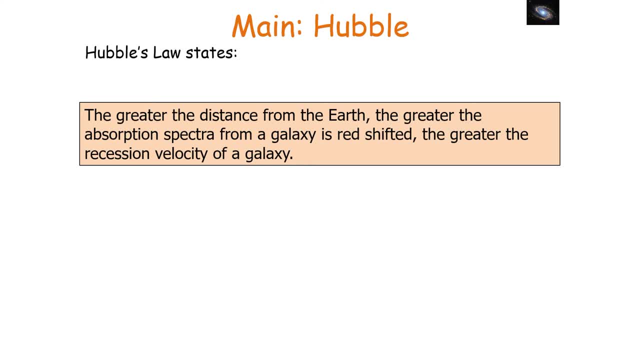 that the greater the distance from the earth, the greater the absorption spectrum from a galaxy is redshifted, the greater the recession velocity of a galaxy, which in equation form is given, which the equation recession velocity is equal to the hubble constant times by the distance from the earth, which is given to you in your examination booklet. now you've got to be able. 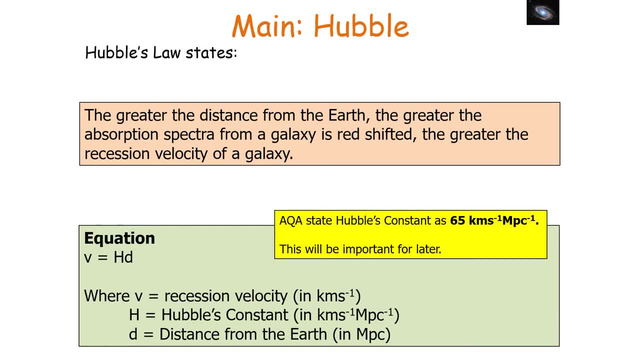 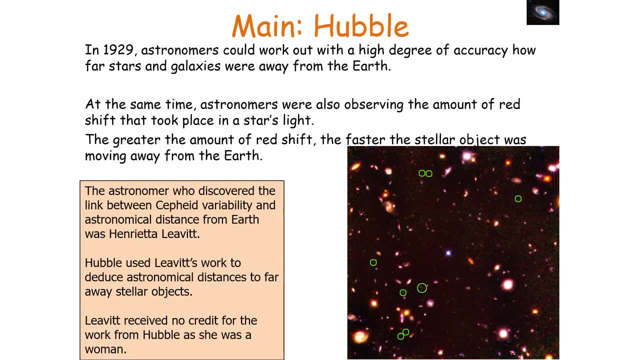 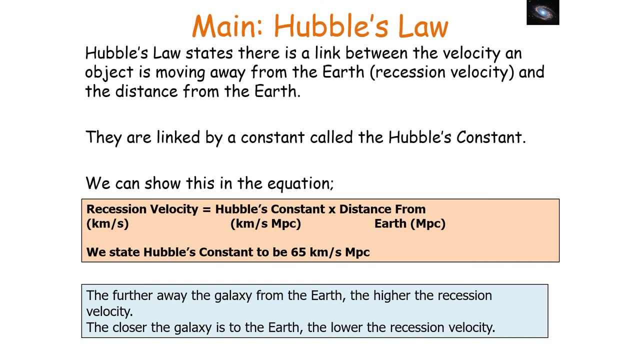 to use this equation, not memorize it now. aqa states that Hubble's constant is 65 km per second per megaparsec. Now it's important to know that, as we move forward here, that the further the galaxy is from the Earth, the higher the recession velocity, whilst the closer the galaxy is. 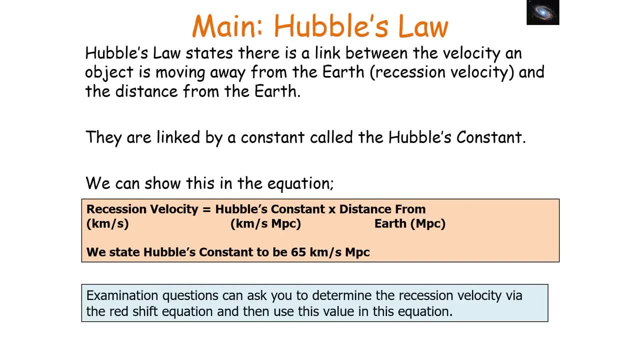 to the Earth, the lower the recession velocity. Now examination questions can ask you to determine the recession velocity via the redshift equation and then use this value in this equation. Now it's important to note that the distance between the Earth and galaxies is very difficult. 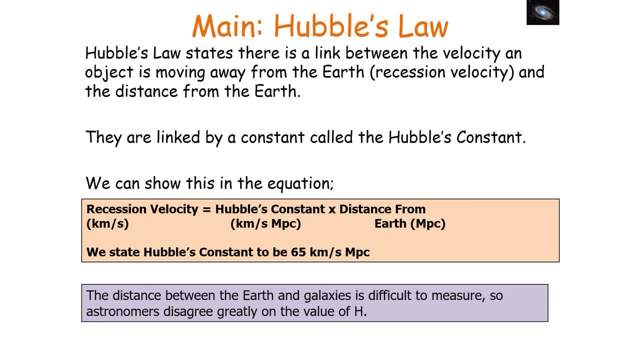 to measure. so astronomers disagree greatly on the value of h. Now. originally Hubble thought that the Hubble constant lied between 50 and 100 km per second per megaparsec. It's now thought that it lies between 65 and 80 km per second per megaparsec. and we now 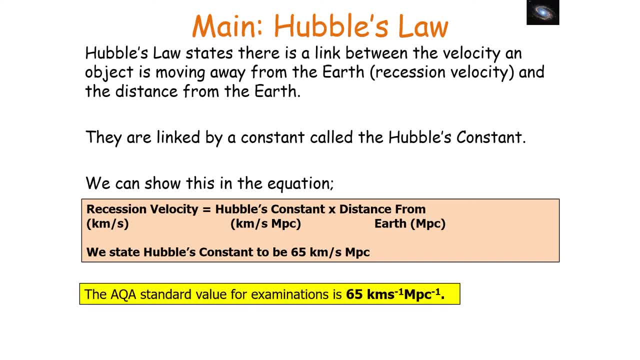 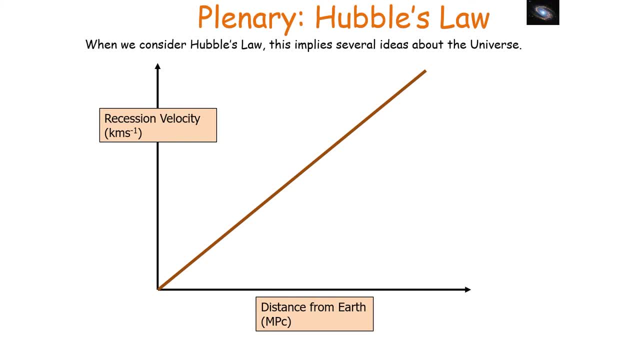 feel it lies at approximately 70.. Now again in the AQA examination, we like to use the standard value of 65 km per second, per megaparsec. Now, when we consider Hubble's law, this implies several ideas about the universe. 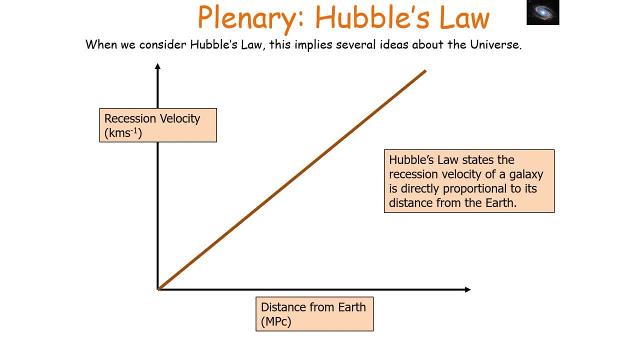 Now Hubble's law states that the recession velocity of a galaxy is directly proportional to its distance from the Earth. Now, in this particular graph, the gradient of the line is the Hubble constant. Now we believe this effect is due to the cosmological redshift. 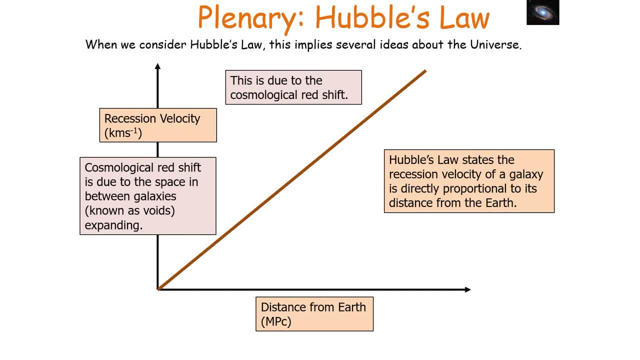 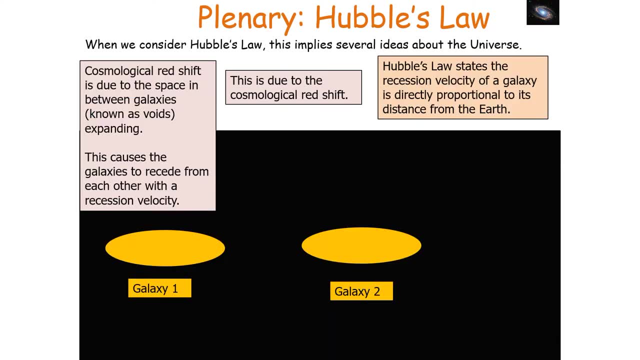 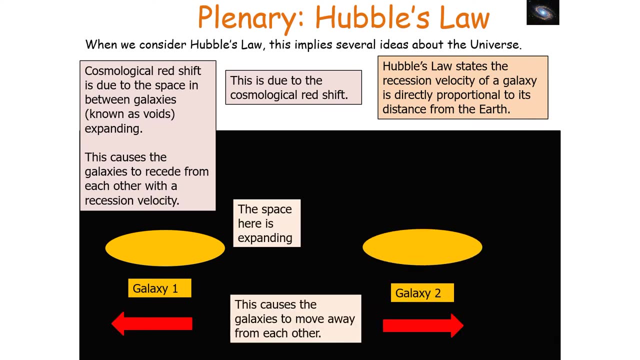 So cosmological redshift is due to the space in between the galaxies expanding, which causes the galaxies to recede from each other with a recession velocity. So if we can imagine galaxy 1 and galaxy 2 here, space in between the two galaxies is expanding. this causes the galaxies to move away from. 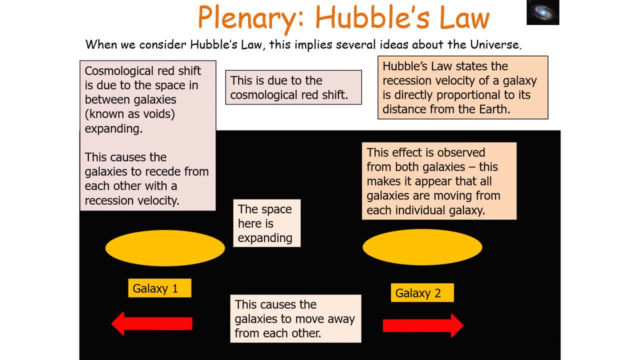 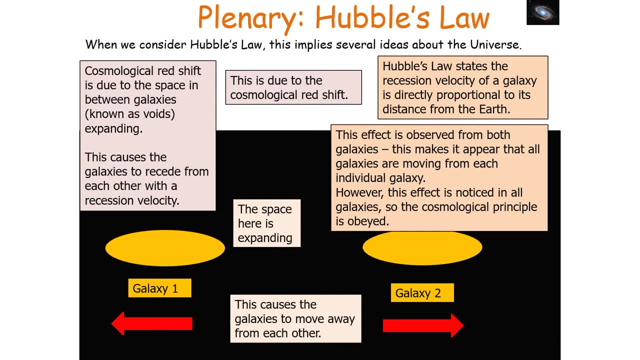 each other. Now this effect is observed from both galaxies, so it makes it appear that all galaxies are moving away from each other. Now this effect is noticed in every single part of the universe. so our cosmological principle: where there is no special place, 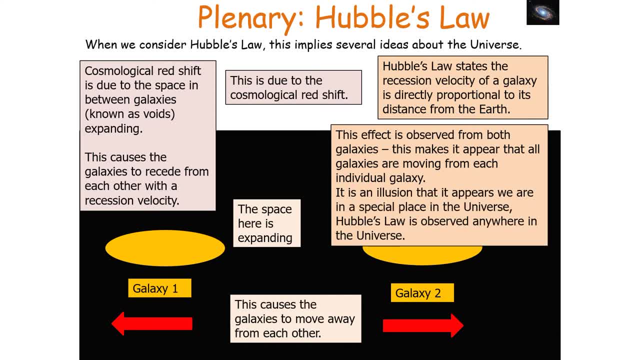 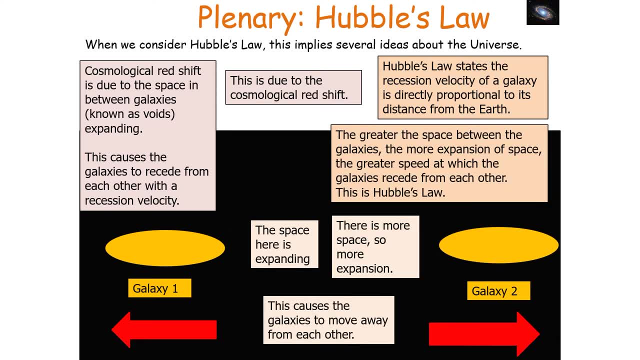 in the universe is still obeyed. It's an illusion where it appears that you are in a special place in the universe. Hubble's law is observed anywhere in the universe. So let's just clarify what Hubble's law is. The greater the space between galaxies, the more the expansion of 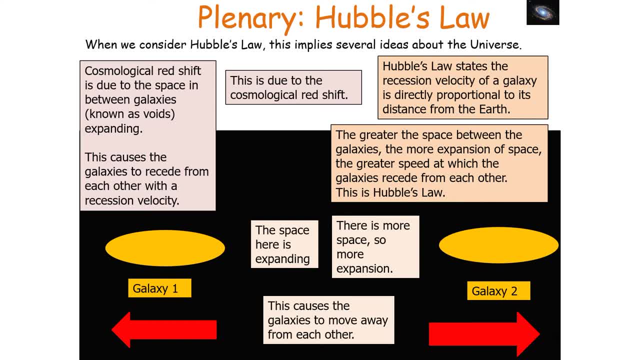 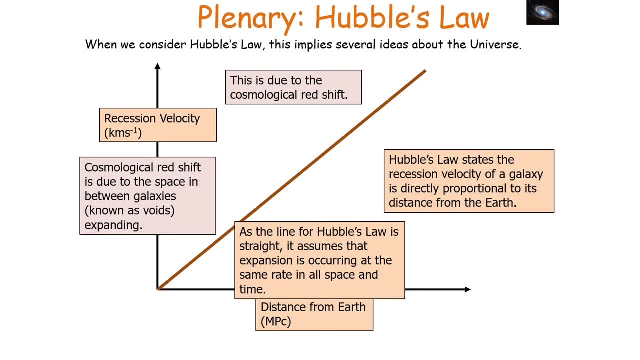 space, the greater the speed at which galaxies recieve from each other. that is Hubble's law. Now, it's important to note that, as this line for Hubble's law is straight, it assumes that the expansion of the universe is occurring at the same rate in all space and all time. 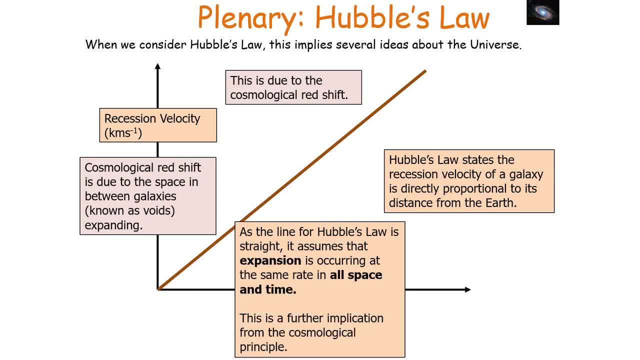 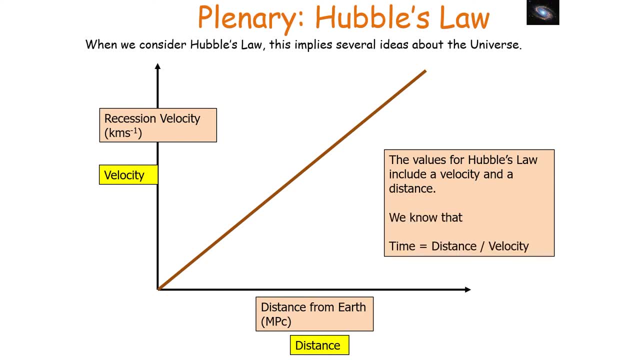 which is a further implication from the cosmological principle. But also we can note that because we have velocity on the y axis and distance on the x axis, we can also work on the velocity on the y axis and distance on the x axis. we can also work on the x axis, we can also work on the. 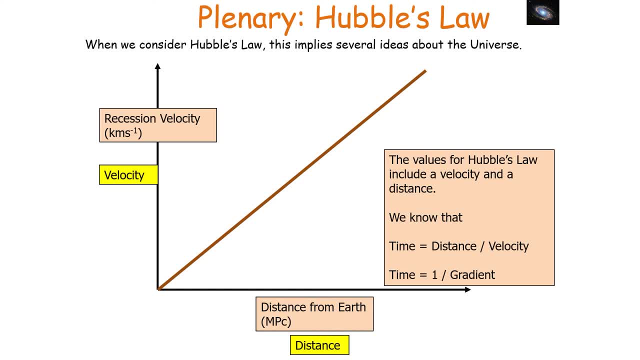 out time because time is equal to distance over velocity. so time in this example is equal to 1 over gradient, where the gradient is the Hubble's constant. So therefore, time is equal to 1 over Hubble's constant. So we use this time to have the first estimate for the age of the universe. 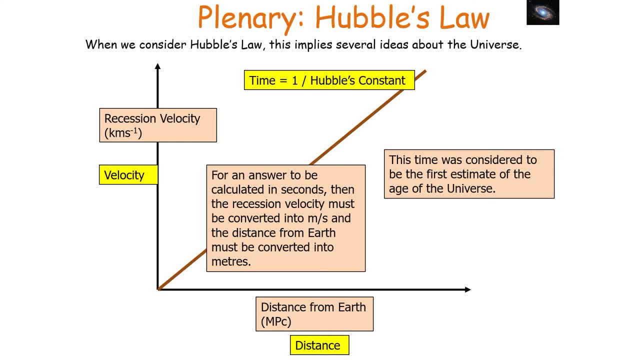 Now for the answer to be calculated in seconds. the recession velocity must be converted into meters per second and the distance from the earth must be converted into meters. So for answers to be calculated into seconds, the units of Hubble's constant must now be in seconds to the minus 1,. 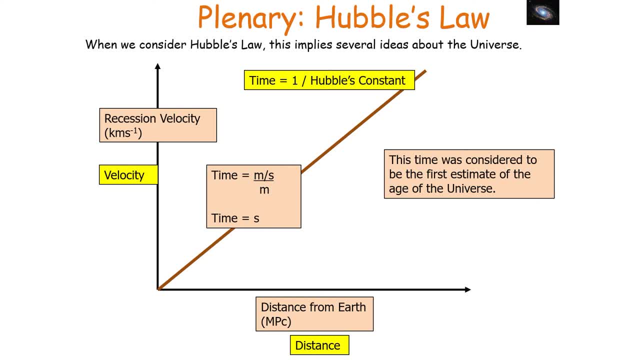 because we have meters per second over meters. that gives our time in seconds. But there are two issues when we calculate a value for the age of the universe with this method. The first issue is it assumes that the universe has been expanding constantly, which we now think not to be true. 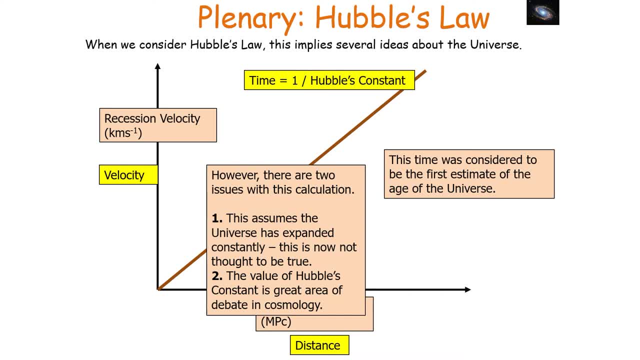 And secondly, the value of Hubble's constant is a great area of debate in cosmology. So this leads to this calculation being an overestimate for the age of the universe, As we think the expansion of the universe is increasing in rate. So we actually now refer to 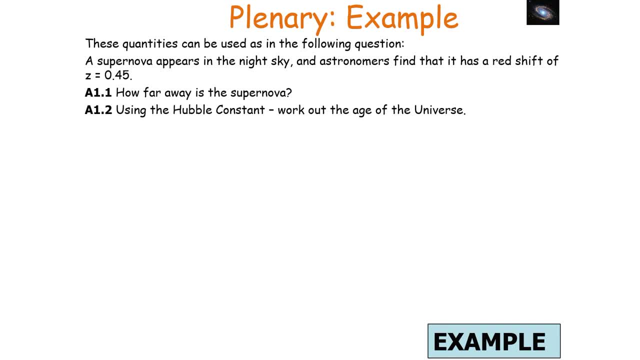 this value as the Hubble time. So let's look at an example question: So how far away is a supernova which has a redshift of z equals 0.45? And can we use this to work out the age of the universe? 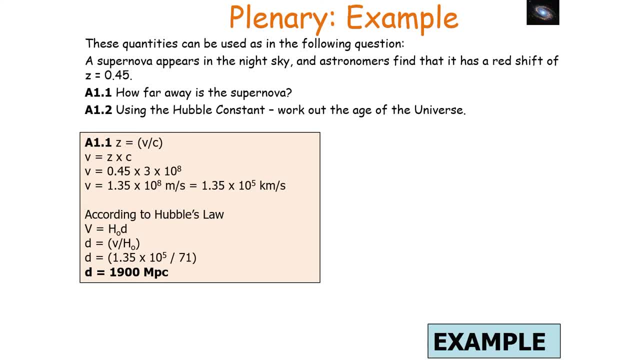 So we say z equals v over c. So therefore we can therefore say: v is going to equal to z times by c. So therefore we can work it out to be 1.35 times 10, to the 5 kilometers per second. Now, as we know, in Hubble's law, v equals hd, d equals v over h. 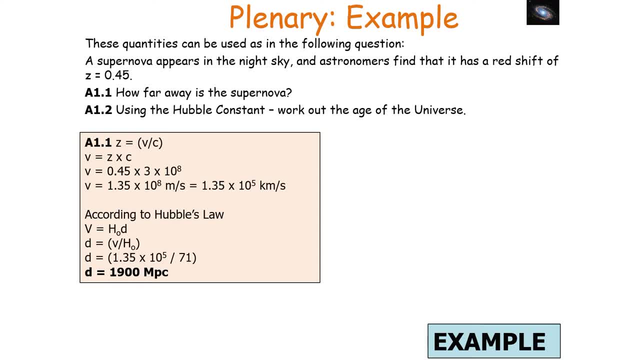 So therefore do 1.35 times 10 to the 5 over 71. The value we're going to use for Hubble's constant in this example. So we get 1900 megaparsecs And therefore we can say that the age of the universe. 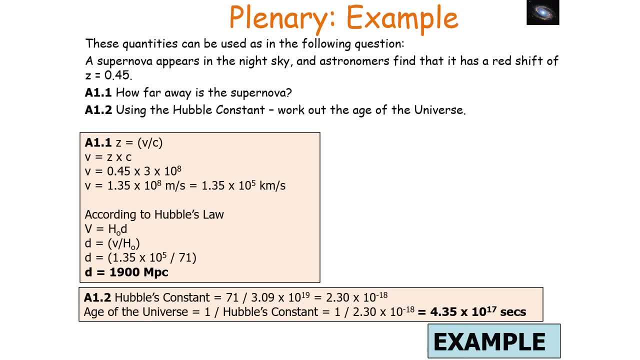 is going to be 1 over Hubble's constant. Now again, we've used Hubble's constant to be 71 in this particular question, So we've got to convert Hubble's constant to seconds to the minus 1, which we can do very quickly. 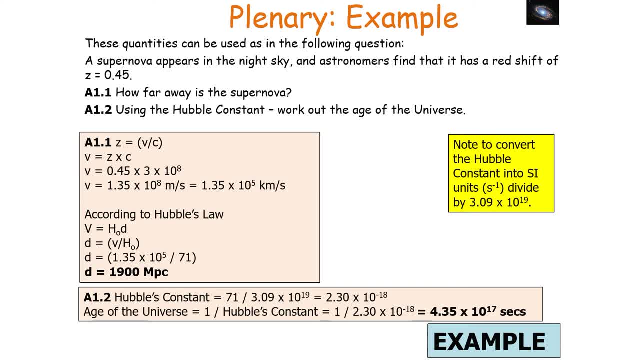 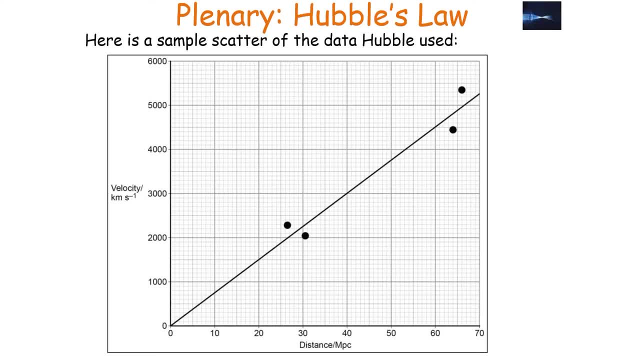 I divide that value by 3.09 times 10 to the 19.. We do 1 over that value and we get 4.35 times 10 to the 17 seconds. Now here's a sample scatter of the data Hubble used Now. the data suggests: 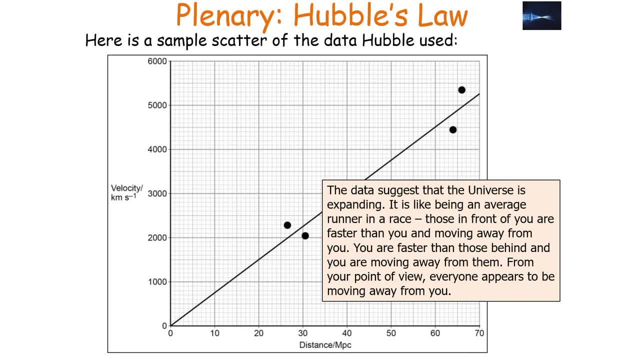 that the universe is expanding. It's like being an average runner in a race: Those in front of you are faster than you and moving away from you, but you are faster than those behind you and you're moving away from them. So, from your point of view, it appears that everyone's moving away from you. 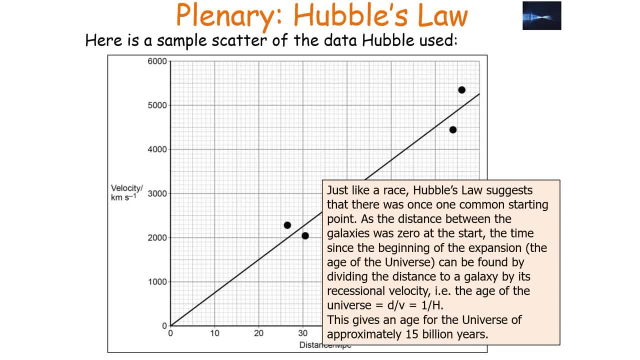 Now I want to note that Hubble's law suggests that once there was one common starting point, So as the distance between the galaxies was zero, the time since the beginning of the expansion, the age of the universe- can be found by dividing the distance to a galaxy by its recession. 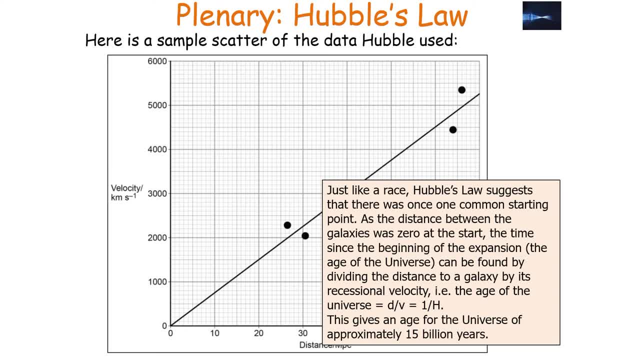 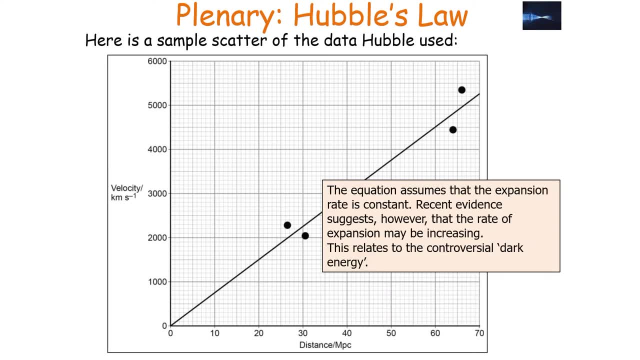 velocity. So it's going to be equal to D over V, 1 over H, which gives an age of about 15 billion years. But this equation assumes the expansion rate is constant. Now recent evidence suggests that the rate of expansion is increasing, which relates to something called dark energy. 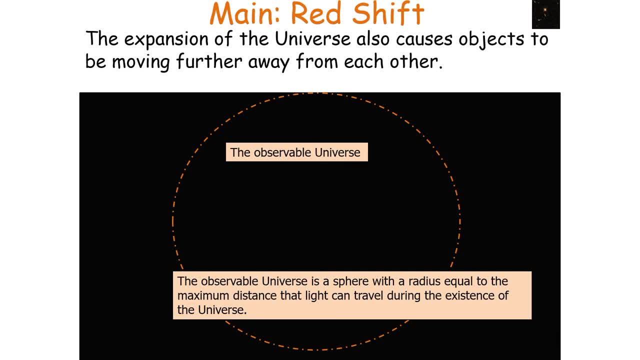 So the expansion of the universe causes objects to be moving further away from each other. So if we consider the observable universe, which is a sphere with a radius equal to the maximum distance that light can travel during the existence of the universe, Now we believe. 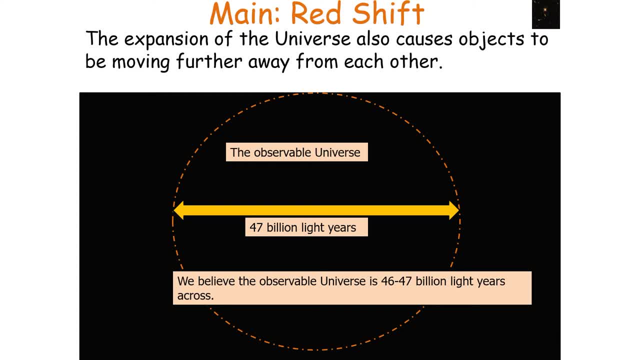 the observable universe is about 47 billion light years across, but we only think the universe is 13.7 billion years old. So the difference in values is due to the expansion of the universe, increasing the size of the observable universe, Because via redshift, Hubble derived the 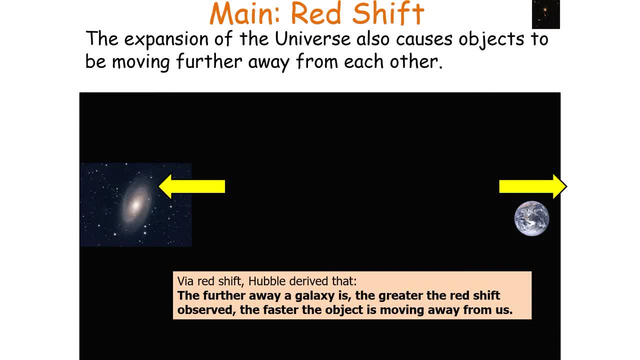 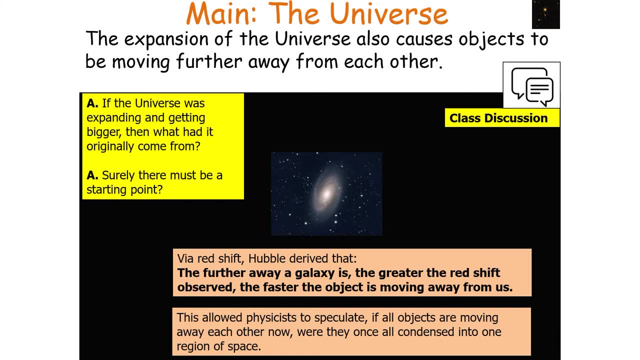 theory that the object moves faster than man, And the further away a galaxy is, the greater the redshift observed, the faster the object is moving away from us. But this allowed physicists to speculate. If all objects are moving away from each other now, were they all condensed? 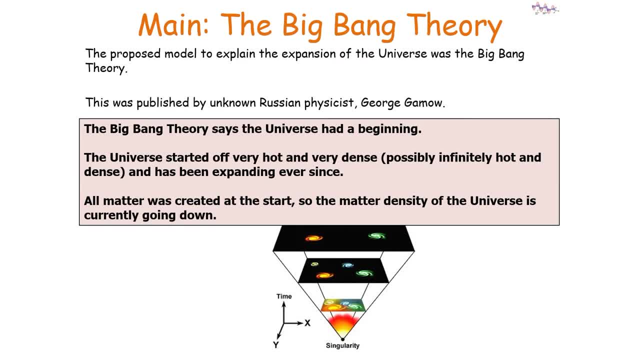 in one region of space. So the proposed model to explain the expansion of the universe from one point was called the Big Bang Theory. So the Big Bang Theory says the universe had a beginning And the universe started off very hot and very dense and has been expanding. 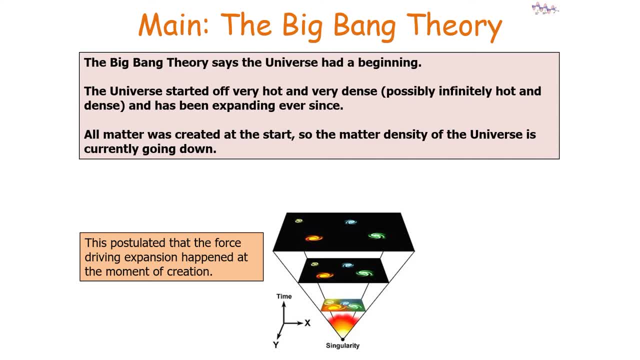 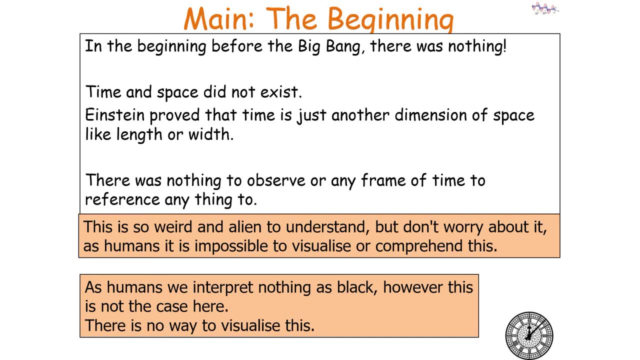 ever since Now. all matter was created at the start of the universe. So this example matter. density of the universe is currently going down. so in the beginning, before the big bang, there was nothing. time and space didn't exist. there was nothing to consider. then the universe comes into. 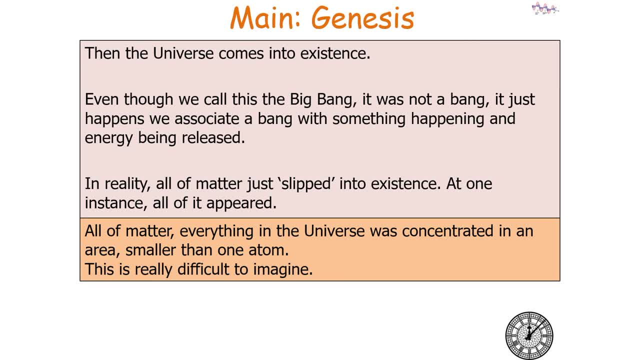 existence. now, even though we call this the big bang, it was. that's just because you associated a bang with something happening and energy being released. in reality, all of matter just slipped into existence in one instance, all of it appeared. so at the big bang, all of time, space, energy and 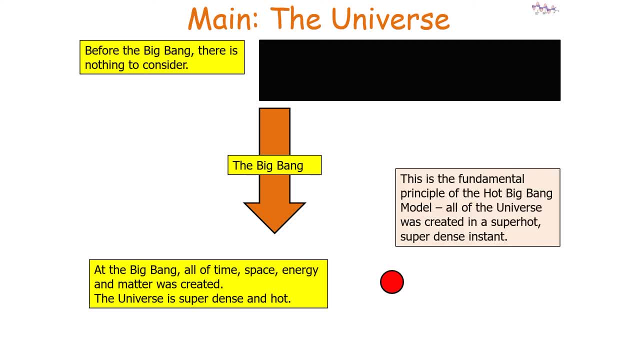 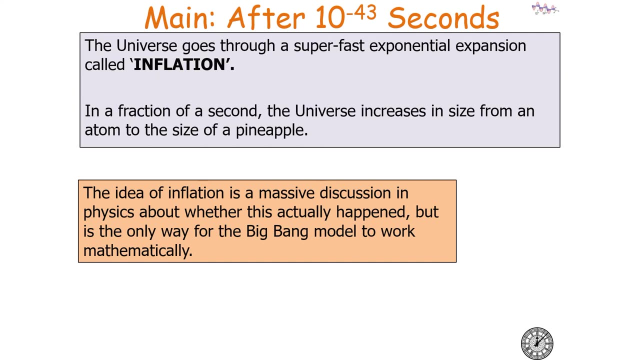 matter was created, the universe was super dense and super hot, which is a fundamental principle of the hot big bang model. all of the universe was created in a super hot, super dense instant. the universe then undergoes a super fast, exponent, exponential expansion, called inflation. so the universe increases in size very quickly and it cools down, as this happens now, we believe. 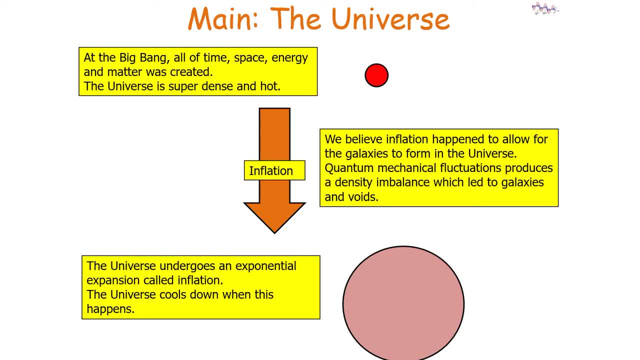 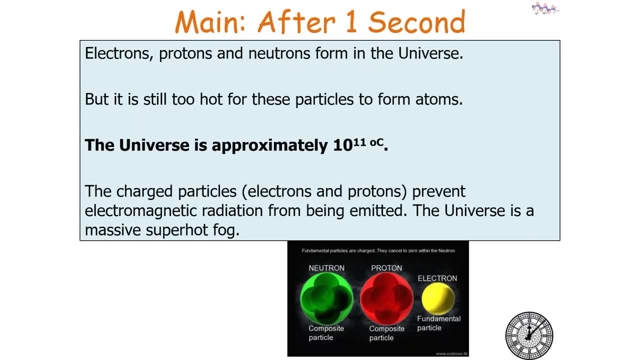 inflation happened to allow for galaxies to form in the universe because quantum mechanical fluctuations produced by the expansion of the universe and the expansion of the universe, a density imbalance which leads to galaxies and voids after one second. electrons, protons and neutrons form in the universe, but the universe is still too hot for the particles to form atoms, so 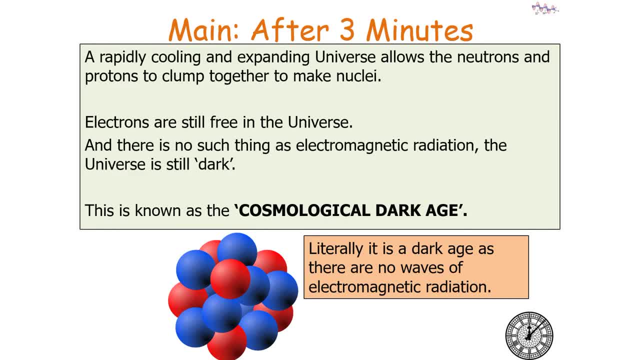 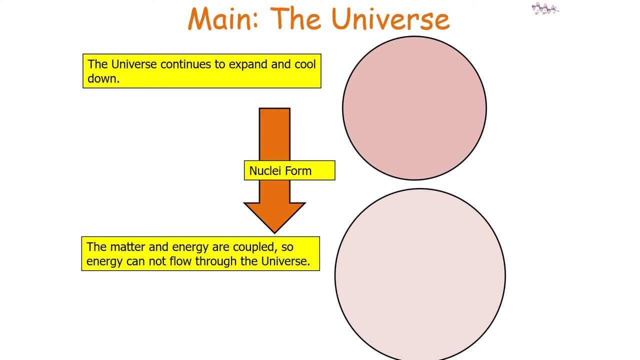 the universe continues to expand and cool down. now, after about three minutes. a rapidly cooling and expanding universe allows neutrons and protons to clump together to make nuclei, but there is still no such thing as electromagnetic radiation. matter and energy are still coupled, so energy cannot flow. 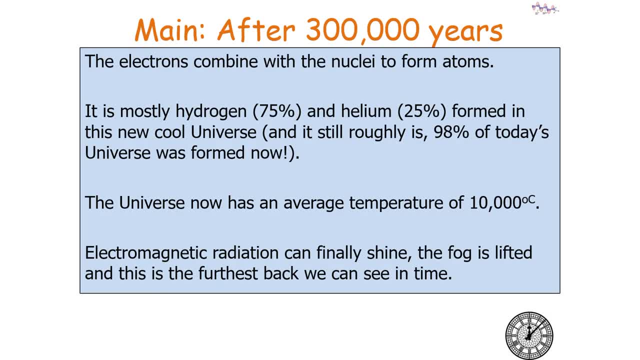 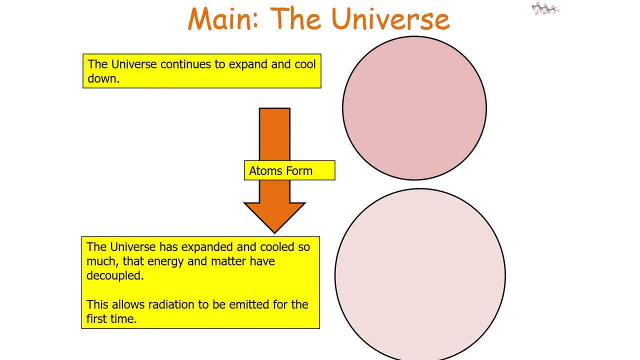 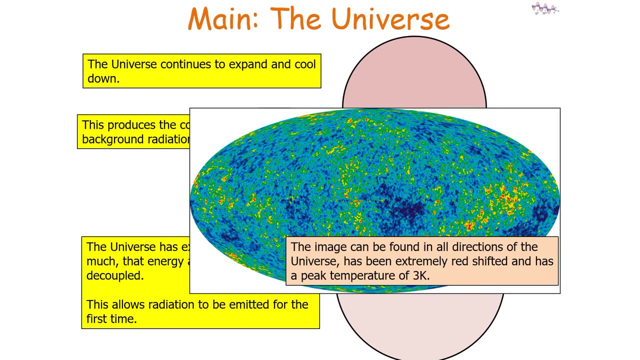 through the universe and after about three hundred thousand years the electrons combine with nuclei to form atoms and now electromagnetic radiation is released for the first time. so this allowed radiation to be released and emitted which we now observe as the cosmic microwave background, so this image can be found in all directions of the universe. it's been extremely red shifted. 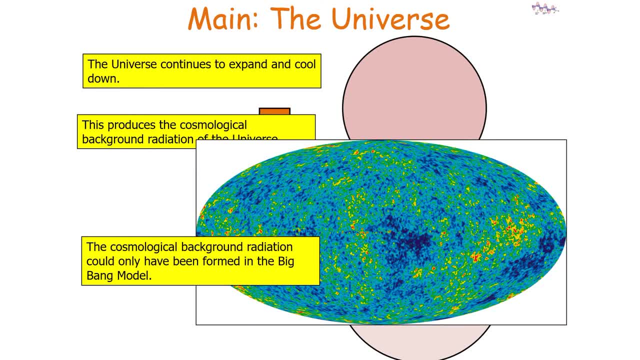 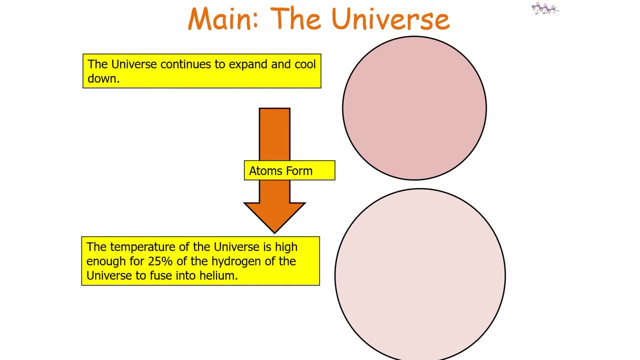 and has a peak temperature of 3 kelvin. now the cosmological background radiation could only have been formed in the big bang model. now the temperature of the universe is higher than the high enough at this point for 25% of the hydrogen of the universe to fuse into helium. These 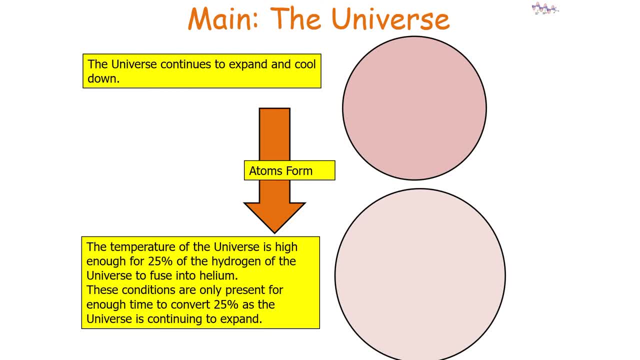 conditions are only present for enough time to convert 25% as the universe continues to expand and cool. The abundance of hydrogen and helium can only be explained by the Big Bang model. So just to clarify before we move on. the cosmological background is an image of the 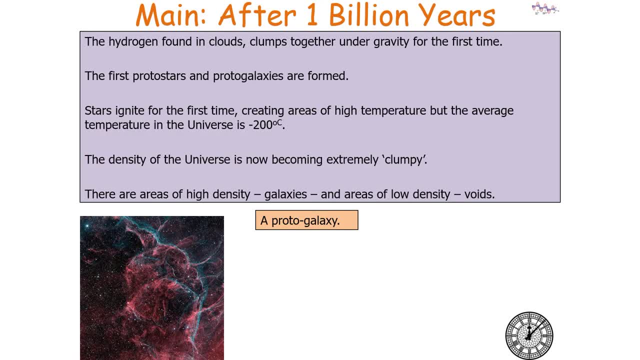 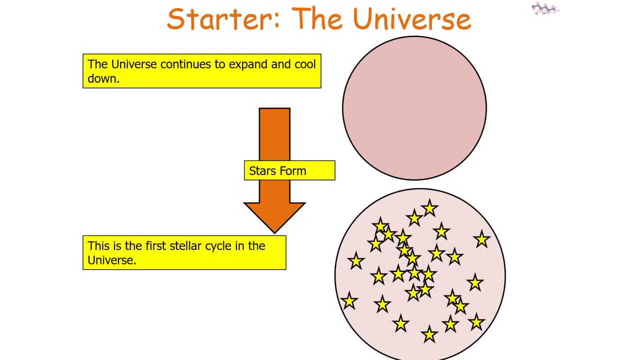 universe aged 300,000 years old. After 1 billion years, the hydrogen found in clouds clumps together under gravity the first time and you get your first protostars and protogalaxies. So we now have our first stellar cycle. This forms massive stars which quickly move through. 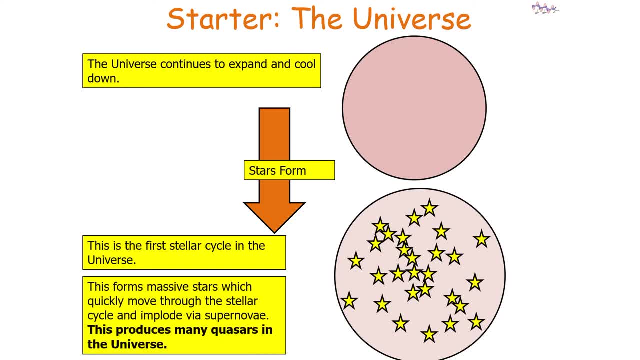 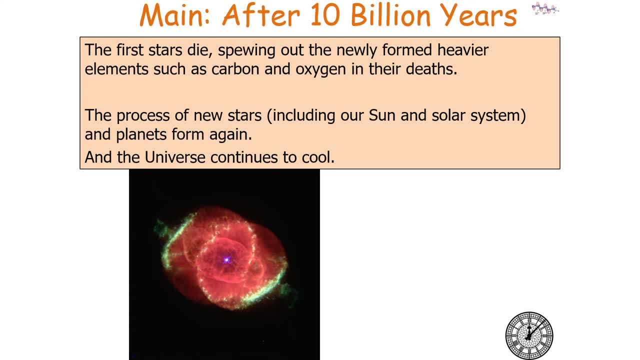 the stellar cycle and implode via supernovae, which produces many quasars in the universe. After about 10 billion years we've now got our first heavier elements produced in those star deaths. The second stellar cycle occurs and the universe becomes more and more clumpy. 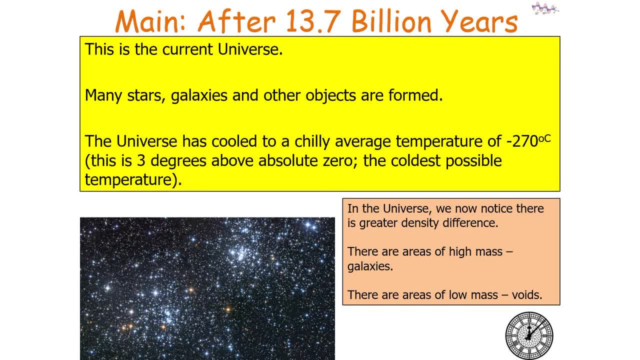 There are regions of galaxies and voids in the universe. So now, 13.7 billion years from now, we've got our first stellar cycle and the universe becomes more and more clumpy. There are regions of galaxies and voids in the universe, So now, 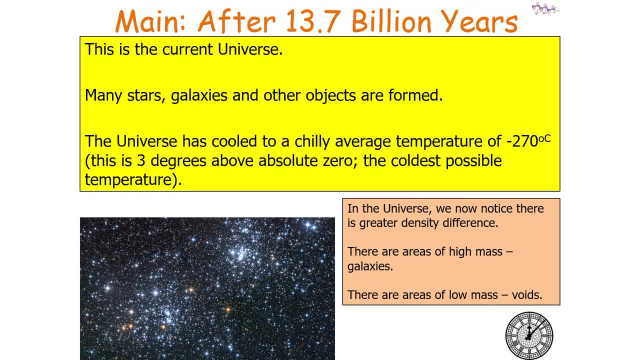 13.7 billion years from now, we have our first stellar cycle and the universe becomes more and more clumpy, with many stars and galaxies and other objects formed. So the universe started off as a hot, very dense universe which was very uniform. Now, 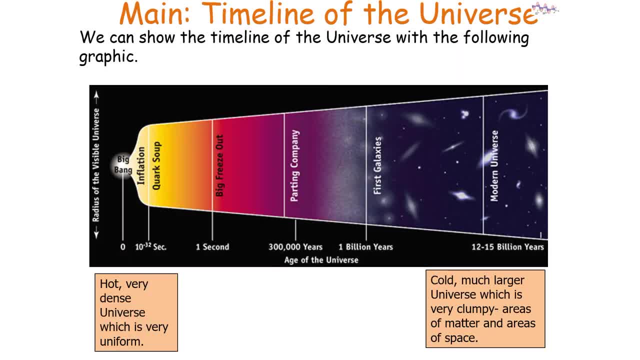 we live in a very cold, very large and very clumpy universe where there is areas of matter and areas of space. So it is very important to remember that the early universe was very hot, very dense and very uniform And, in addition, the observable universe is very 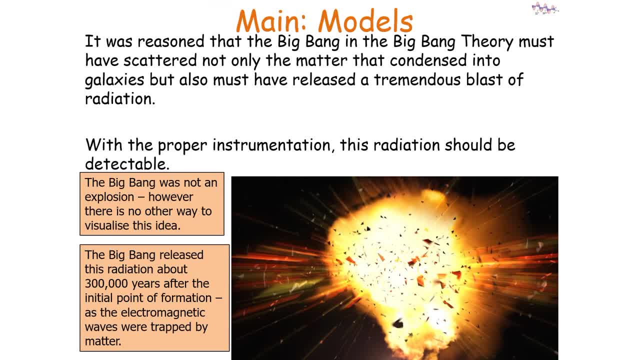 small when it was very, very young. So I'm sorry these start instead of minutes. know that the Big Bang occurred Now. the Big Bang was not an explosion, but there's no other way to visualize this idea. Now. the Big Bang released radiation about 300,000 years after the initial. 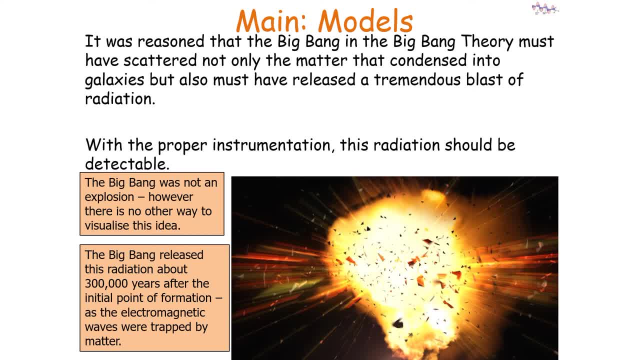 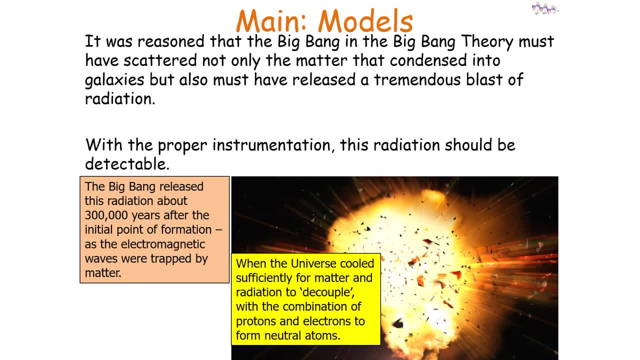 point of formation. as before then, electromagnetic waves were coupled with matter. So when the universe cooled sufficiently for matter and radiation to decouple, the combination of protons and electrons formed neutral atoms. So this radiation is found in all directions we observe. it's cosmic and it can be considered to have its own blackbody radiation curve. 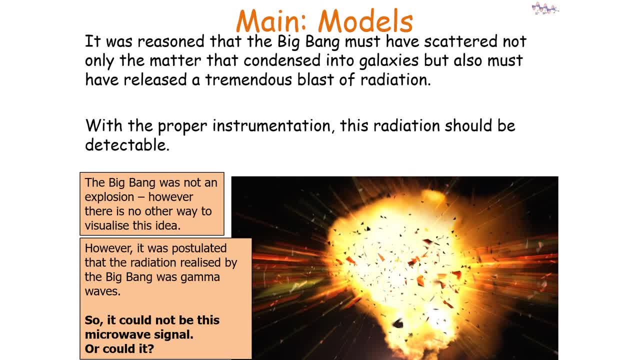 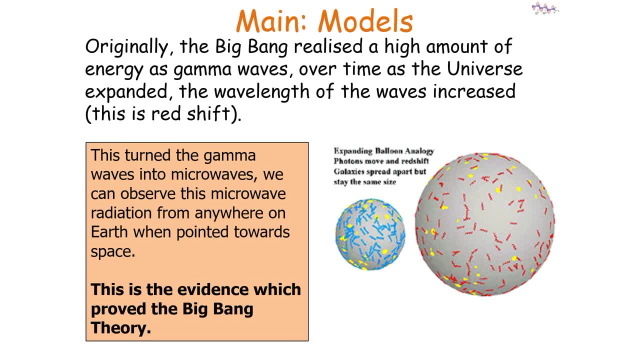 Now this curve has a peak temperature of 3 Kelvin. Now. it was originally released as gamma waves, but over time, because as the universe has expanded and expanded and expanded, these gamma waves have turned into microwaves, So they now have formed the cosmological microwave. 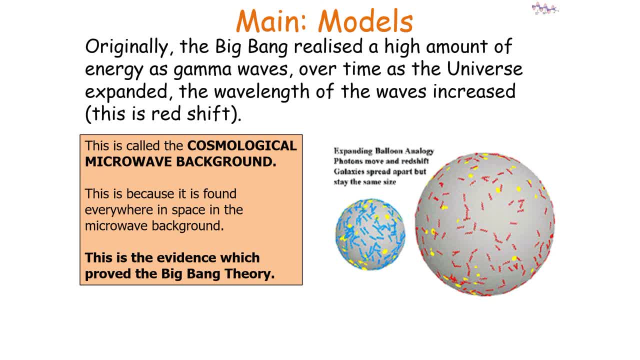 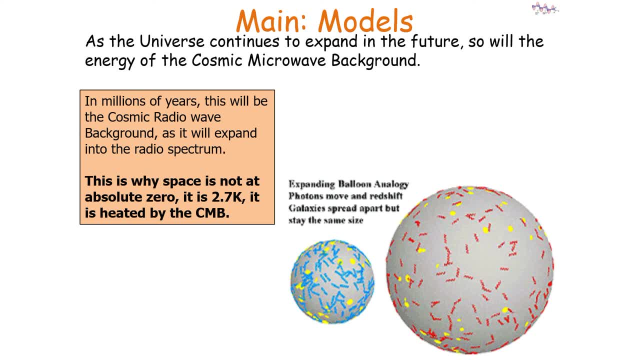 background. So this is evidence which provides evidence for the Big Bang theory. So in millions of years, as the universe continues to expand, it will become the cosmic radiowave background, And this is why space is not found to be at absolute zero: It's at 2.7 Kelvin. 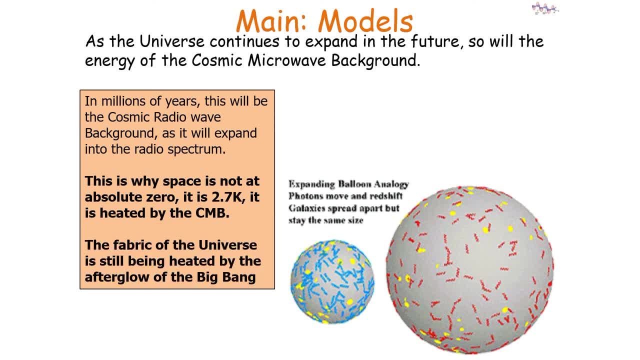 because it's heated by this cosmological microwave background. The fabric of our universe is still being heated by the afterglow of the Big Bang. Now, like I said before, it can be considered the universe has its own blackbody radiation curve with a peak temperature of 2.7 Kelvin. 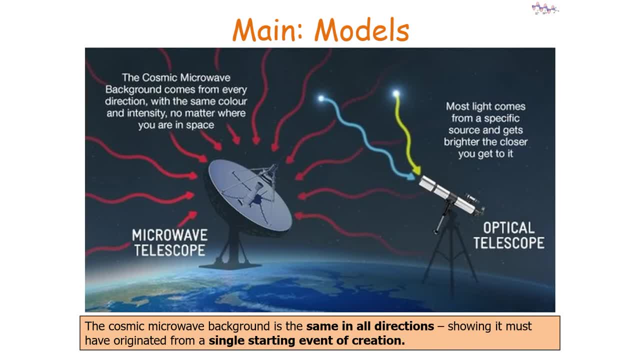 So the cosmological microwave background is the same in all directions shown and must have been coming from a single starting point of the Big Bang. So the cosmological microwave background is the same in all directions shown and must have been coming from a single starting point of the Big Bang. So the cosmological 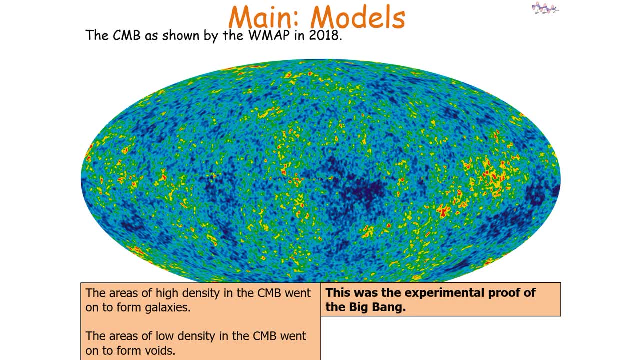 microwave background is the same in all directions shown and must have been coming from a single starting point of the Big Bang. Same with a cold humidity of 8-10 degrees when we see these particular images. So the other piece of evidence for the hot Big Bang. 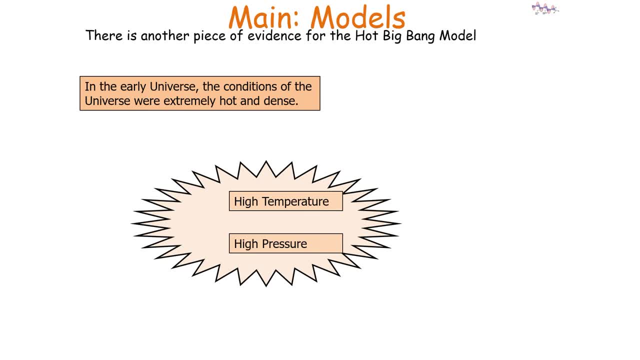 model is that the conditions of the universe were extremely hot and extremely dense, So these conditions were high enough for fusion to occur. So this caused the first protons, hydrogen, to fuse into helium. This meant the that the early universe was made of hydrogen. 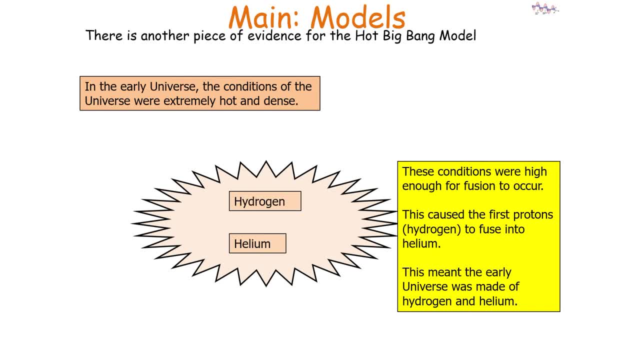 and helium. So we can now see we're producing hydrogen and helium, but overtime the universe cooled. when it exploded, It lets the first hizo gloves cool down, will allow for fusion of hydrogen and helium. but over time, this is they themselves, would be storage and this is it a process they can Fake to produce grandfathered. 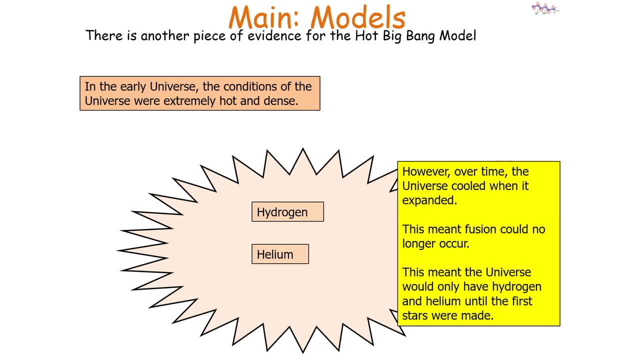 expanded, So this meant fusion could no longer occur. This meant that the universe would only have hydrogen and helium until the first stars were made. Now the Big Bang model predicts, at the rate of expansion, that there was only enough time to make 25% of the universe into helium and 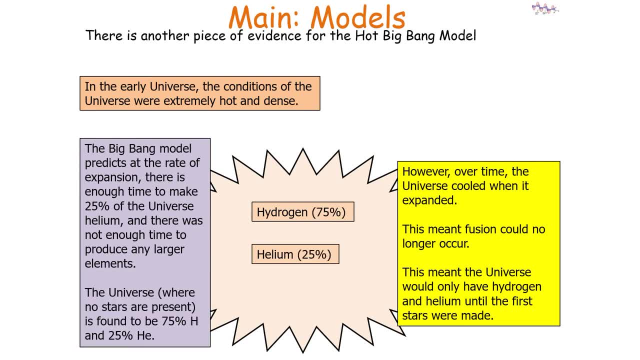 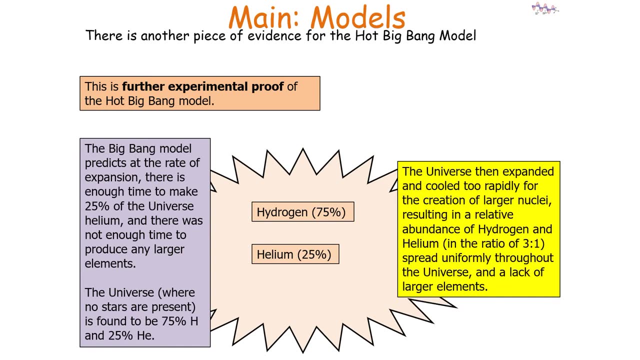 there was no time to produce any larger elements, So the universe in theory should be 75% hydrogen and 25% helium, which is what we observe. So this is further experimental proof of the hot Big Bang model. Now the universe expanded and cooled too rapidly for any creation of large nuclei and 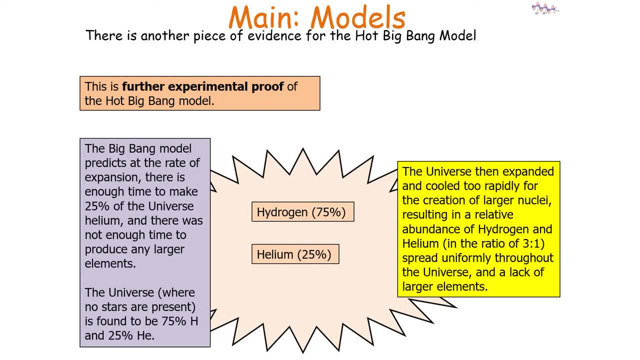 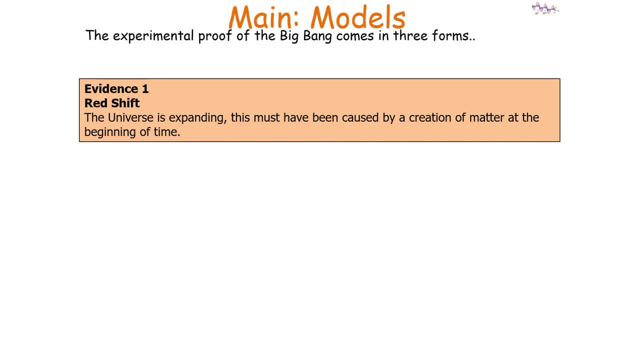 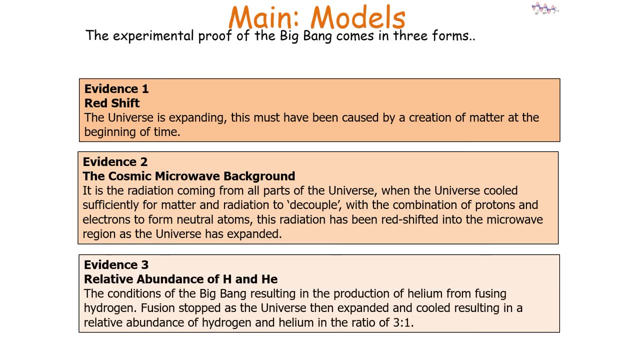 resulted in the relative abundance of hydrogen and helium at a three to one ratio, spread uniformly through the universe which, as we said before, is consistent with observation. So proof of the Big Bang comes in three forms. Evidence one: redshift. Evidence two: the cosmological microwave background. 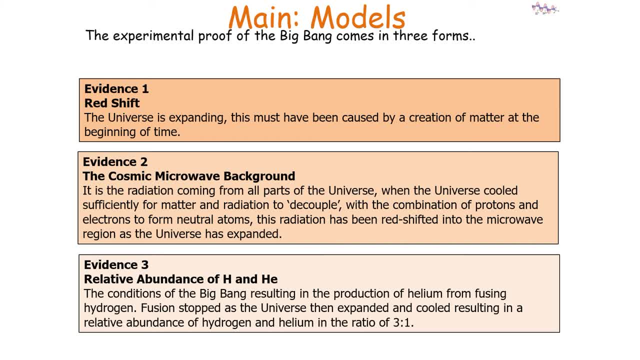 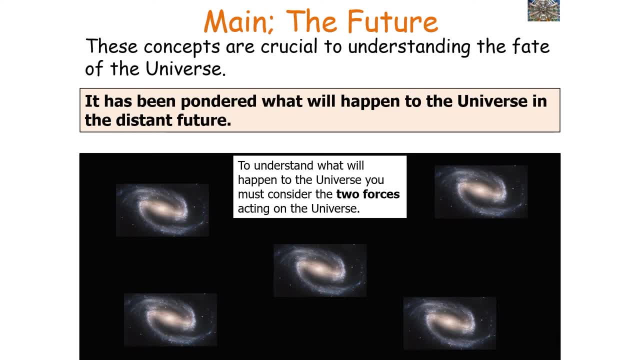 and evidence three, the relative abundance of hydrogen and helium. Now, the idea of the Big Bang taking place in the universe is that it's not just the universe but the universe itself. So the idea of the Big Bang taking place allows us to consider how the universe began, but we've also 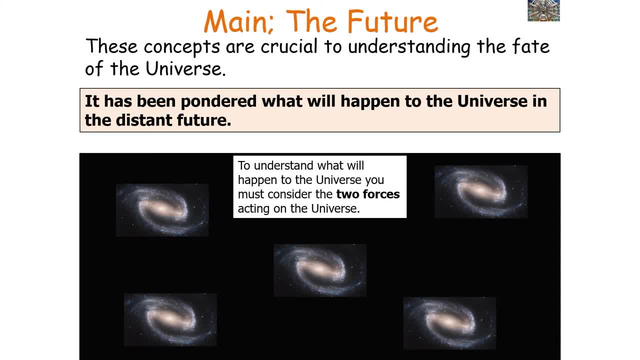 pondered what will happen to the universe in the distant future. So to understand what will happen, we've got to consider the two forces acting on the universal scale. So we've got gravitational attraction pulling the universe inwards, caused by dark matter and visible matter of the universe. 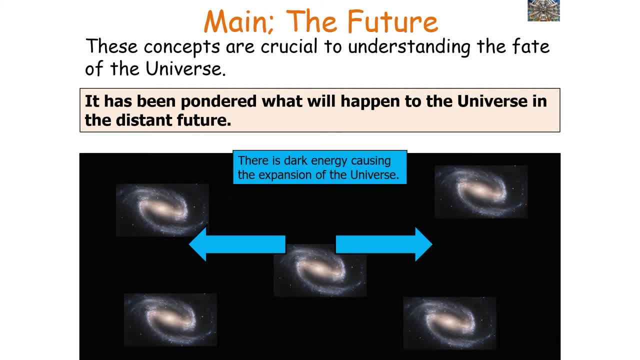 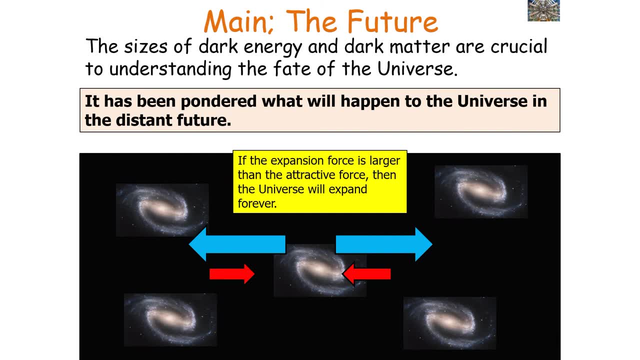 and we've got dark energy causing the expansion of the universe. So the relative sizes of dark energy and dark matter will lead to how the universe will evolve in the distant future. If the expansion forces are larger than the attractive force, the universe will expand forever. This is called the open. 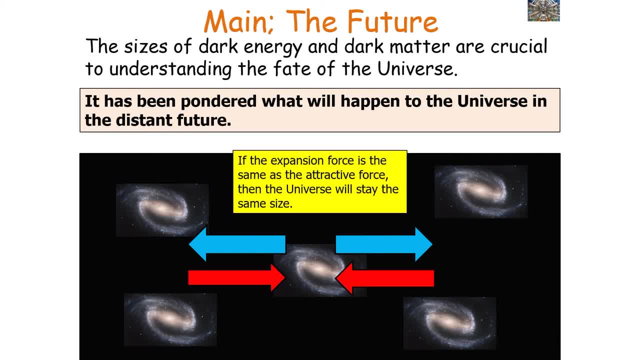 universe. Now, if the expansion force is the same size as the attractive force, the universe will stay the same size. This is called the flat universe. And if the expansion force is smaller than the attractive force, then the universe will decrease back to a singularity. This is called 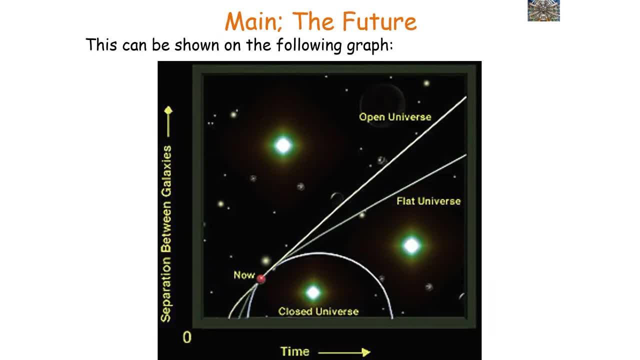 the closed universe. So you've got three possible options of how the universe will evolve Now. for a long time, astrophysics didn't know which model the universe will take. However, scientists have been able to do this by observing distant standard candles in our own universe. 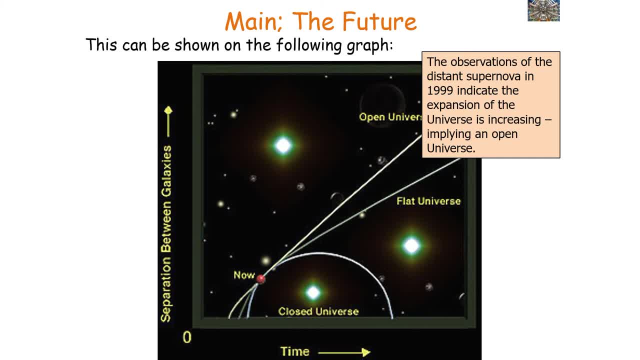 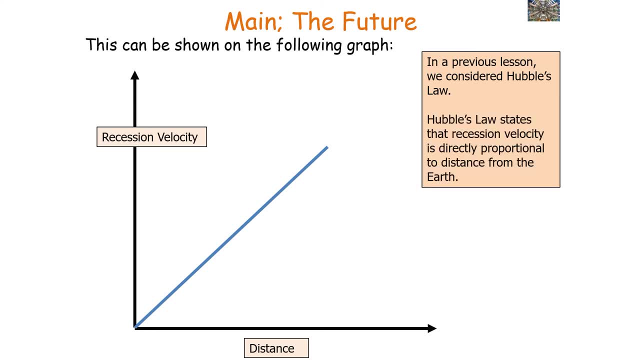 So the observations of distant supernovae in 1999 indicate the expansion of the universe is increasing, implying an open universe. So if we consider our Hubble's law graph, as we know, Hubble's law states that recession velocity is directly proportional to the distance. 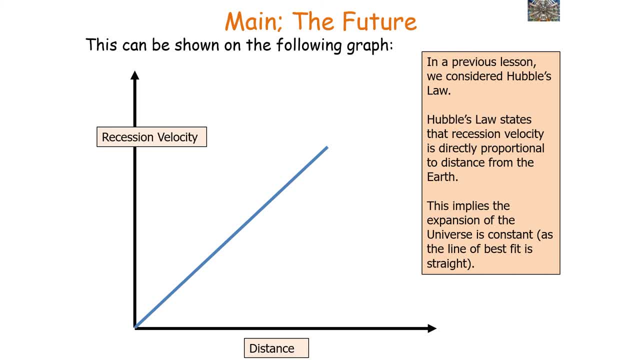 from the earth, implying the universe has an expansion rate which is constant. we've got a straight line of best fit, So we can extrapolate the trend for more distant objects. So in 1999, we measured the most distant type 1a supernovae. Now, if Hubble's law is to be obeyed, they should. 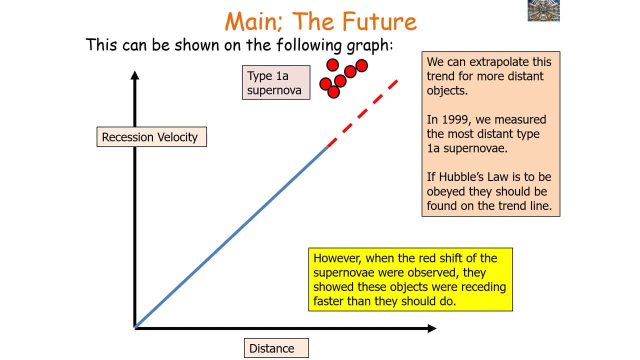 be found on the trend line here. However, when the redshift of the supernovae were observed, this showed that the objects were receding faster than they should do, So they were redshifted more than we expected. So this implies that the Hubble's law graph trend is increasing This. 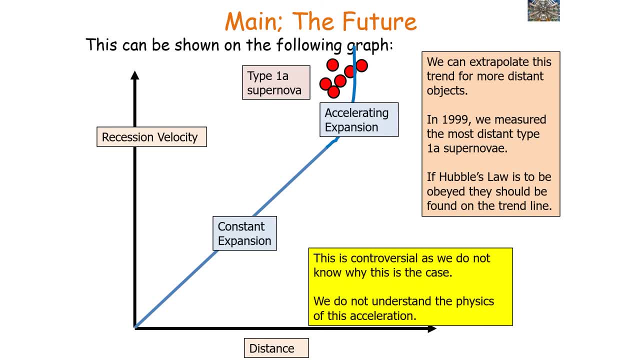 implies that the expansion rate of the universe is accelerating. Now, this is controversial, as we don't know why this is the case. We don't- we don't- understand the physics of acceleration. Now, this conclusion was further confirmed with redshift observed from quasars. 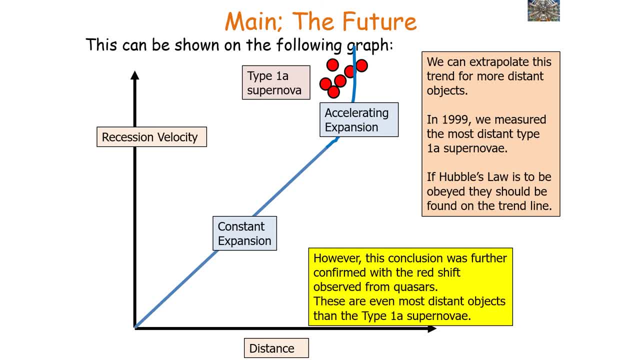 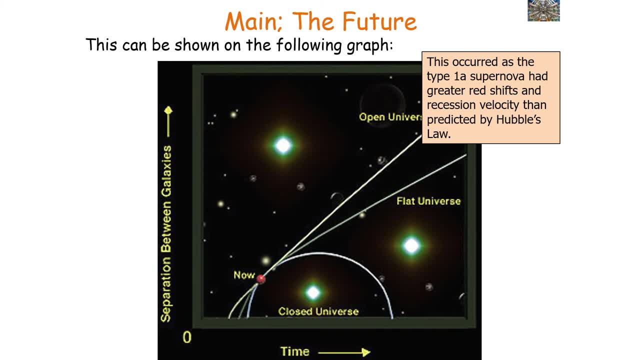 which are even more distant objects than the type 1a supernovae observed in 1999.. So just to clarify, the type 1a supernovae had greater redshifts than predicted by Hubble's law, indicating expansion of the universe is not constant, rather it is accelerating. Now this is controversial as the 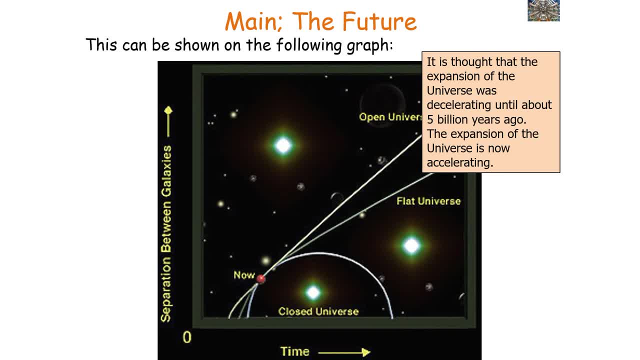 concept of dark energy is not fully understood. It's thought that the expansion of the universe was decelerating until about 5 billion years ago. The expansion of the universe is now accelerating. Now, dark energy is accepted to exist in the universe, according to current thinking, but we don't know its mechanism. 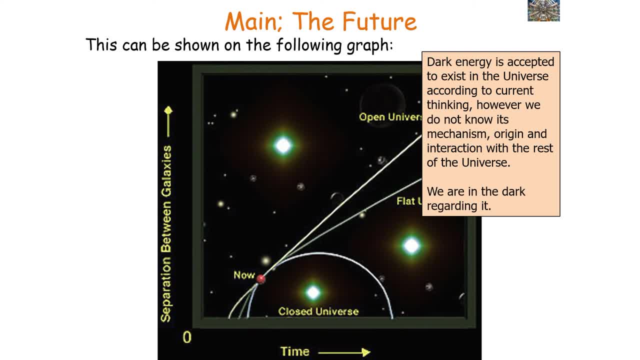 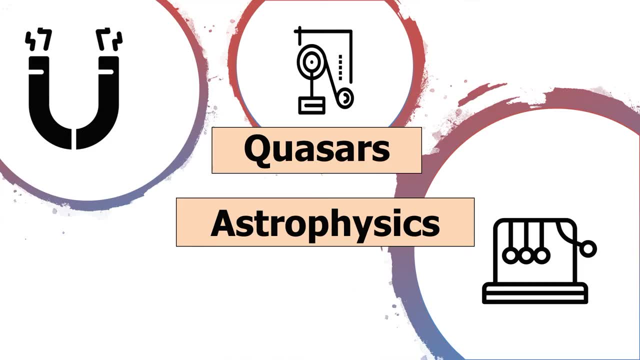 origin or interaction with the rest of the universe. We are in the dark regarding it. Now. we are unsure as to how the universe will evolve, because we're close to the start of the universe. The next thing to look at are quasars. Now, quasars are only observed in the distant. 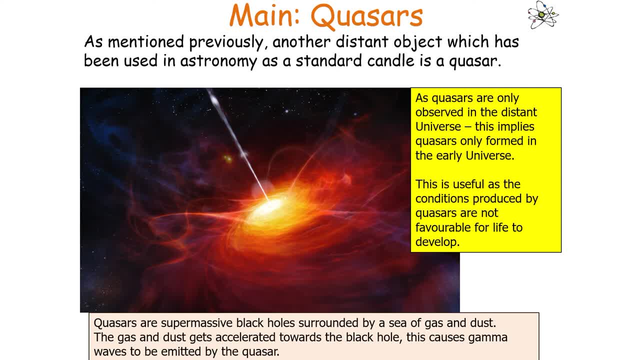 universe, implying that they were only formed in the early universe, which is very, very useful, as they are not a known fact. The conditions produced by quasars are not favourable for life to develop because quasars are supermassive black holes surrounded by a sea of gas and 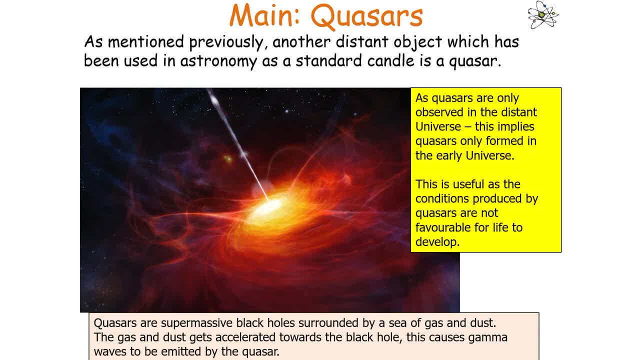 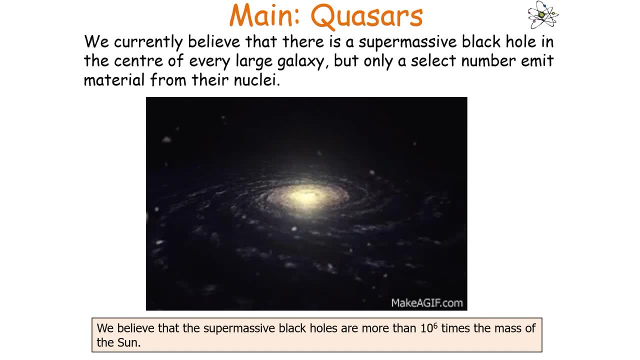 dust. The gas and dust get accelerated towards the black hole, causing gamma waves to be emitted by the quasar. So we currently believe that there's a supermassive black hole in the centre of every galaxy, but only a select number emit material from their nuclei. So we believe that 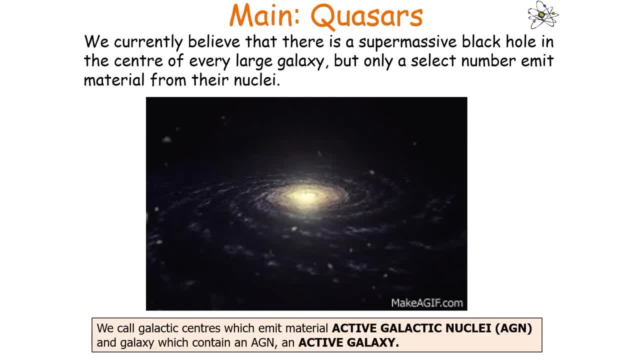 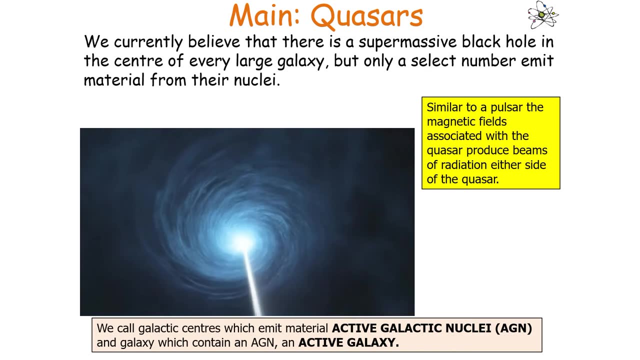 there's supermassive black holes, ten to the six times more massive than that of the sun. Now call galactic centers which emit material active galactic nuclei and the galaxies which contain an AGN an active galaxy. Now we currently believe that there's a supermassive black hole in the center of every large galaxy, with only a 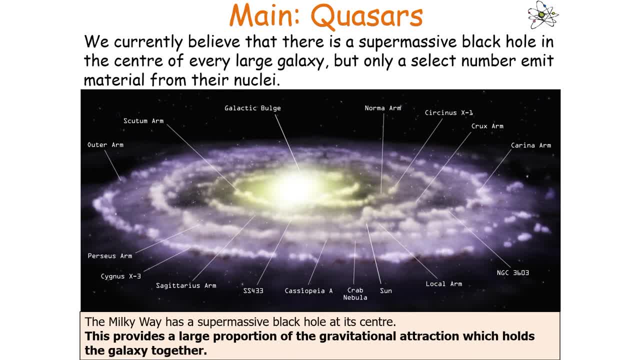 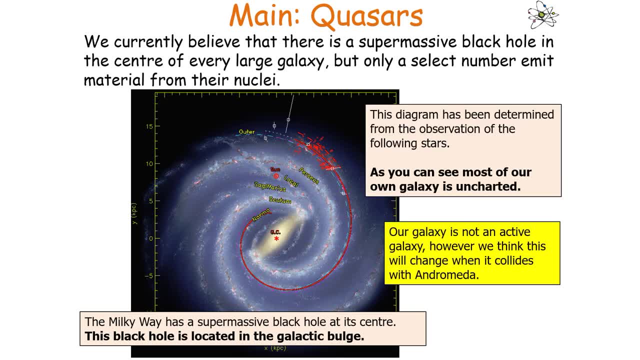 select number emit material from their nuclei. Now the Milky Way has a supermassive black hole at its center which, you can see, is located in the gravity in its own galactical bulge. but our galaxy is not an active galaxy as we think this will. 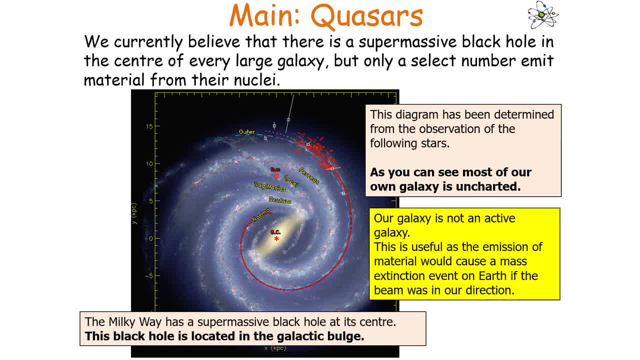 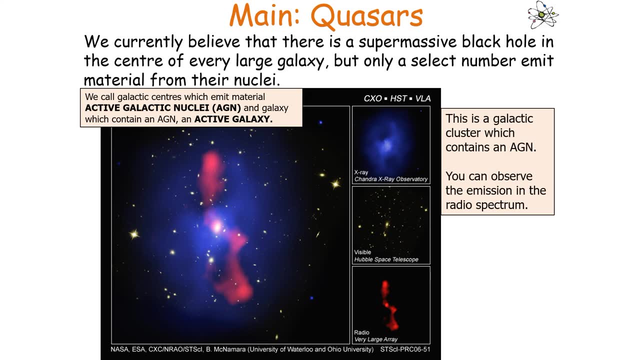 we think this could change when it collides with the Andromeda galaxy. Now it's useful that our galaxy is not an active galaxy, as the emission of material will cause a mass extinction event on the earth if the beam was in our direction. Now this image shows us a galactic cluster which contains an AGN. 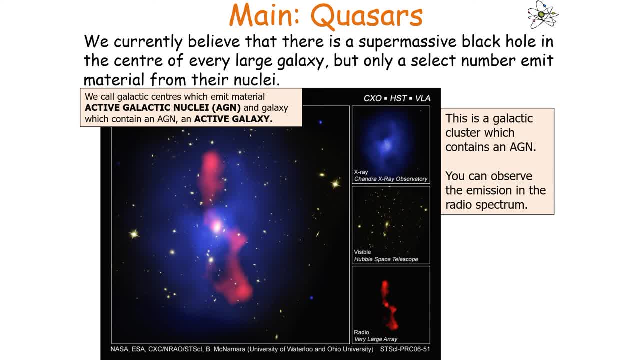 Now you can observe the emission in the radio spectrum. Now that's a very important idea, because quasars and AGN are very, very bright radio source emitters. Now AGN do not have the same power as the radio source emitters. Now, that's a very important idea, because quasars and AGN are very, very bright radio source emitters. Now AGN do not have the same power. 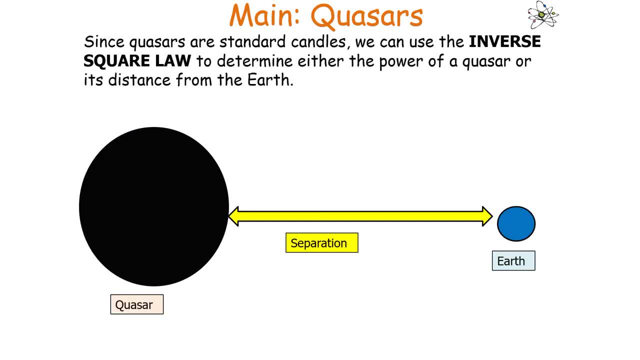 as quasars, but they're still very, very powerful. Now, since quasars are standard candles, we can use the inverse square law to determine either the power of a quasar or its distance from the earth. Now, previously we'd stated that the brightness of an object observed on the earth is dependent on the intensity and 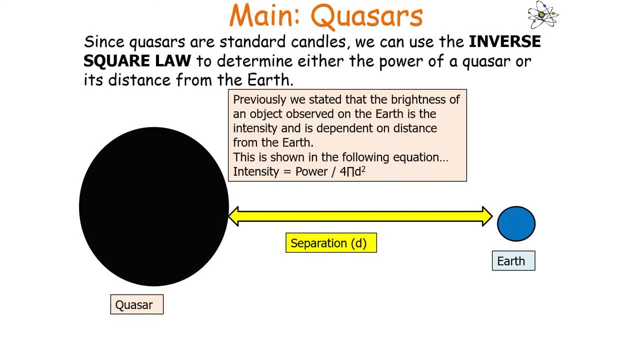 the distance from the earth. So we can show through the following equation that intensity is equal to power over 4 pi D squared, where D is the separation between the object and the earth. So therefore, power is equal to intensity times by 4 pi D squared. So when a quasar has the same 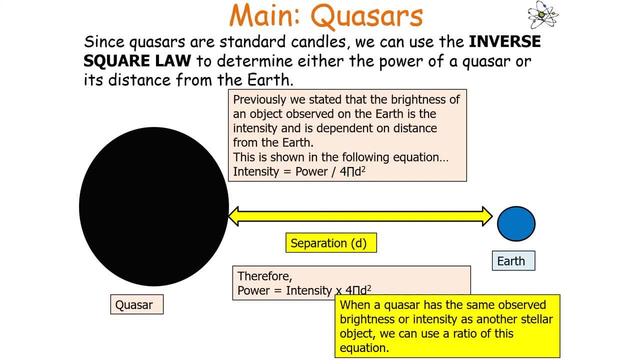 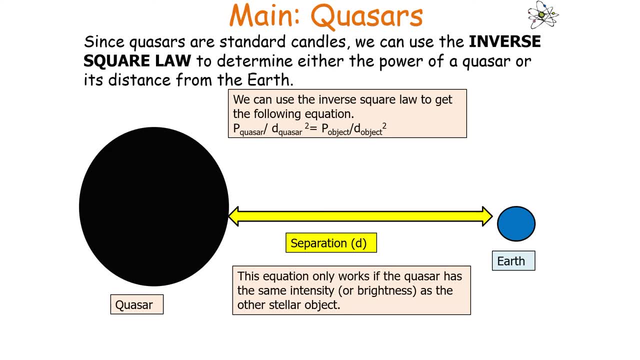 observed brightness or intensity as another stellar object. we can use a ratio of this equation, But this equation will only work if the quasar has the same intensity or brightness as the other stellar object. So we can say the power of the quasar over the distance to the quasar squared is equal to the power of 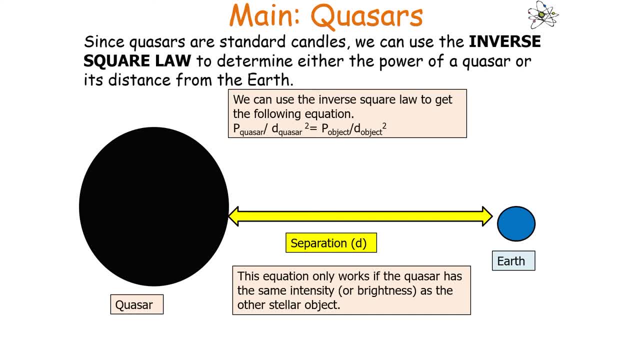 the other object divided by the distance to the other object squared. So because the intensity is the same on both sides of the equation, it can cancel out. So you can say here that the power of the quasar over the power of the object is equal to the distance to the quasar divided by the 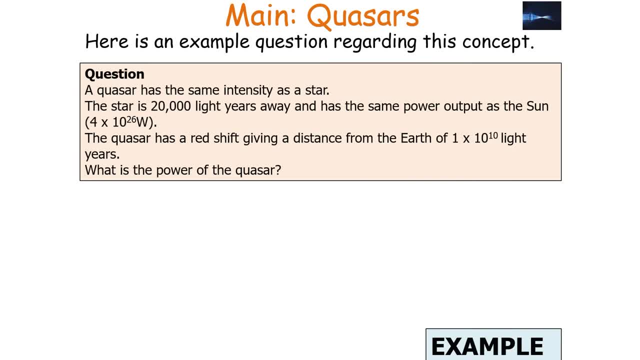 distance to the object squared. So let's look at an example question regarding this concept. A quasar has the same intensity as a star. The star is 20,000 light years away and has the same power output as the Sun. The quasar has a red. 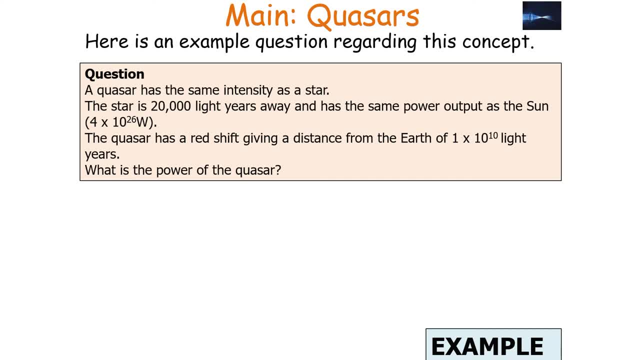 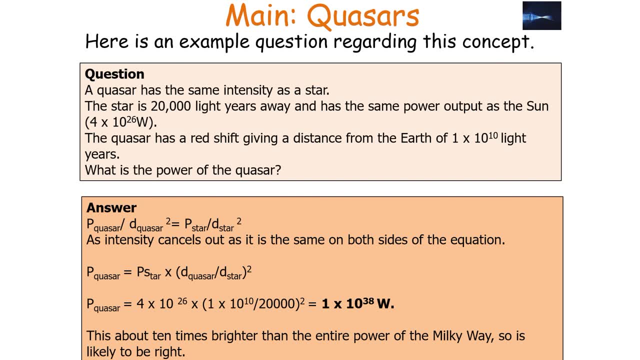 shift, giving a distance from the earth of 1 times 10 to the 10 light years. So what is the power of the quasar? Well, we know that the intensity cancels out because it's the same on both sides. So the power of the 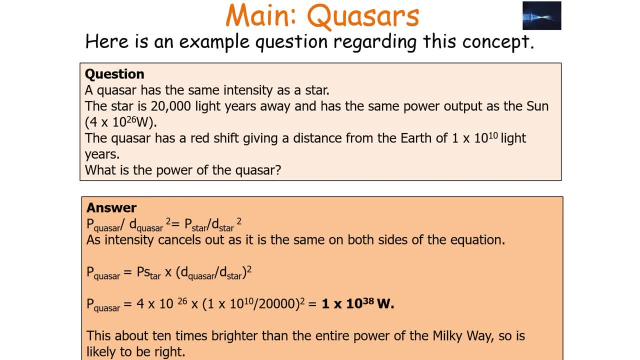 quasar over the distance to the quasar squared is equal to the power of the star over the distance to the star squared. So we can rearrange that and make power of the quasar the subject of your equation. Pop all your values in, work it through and you get an answer of 1 times 10 to the 38 watts. 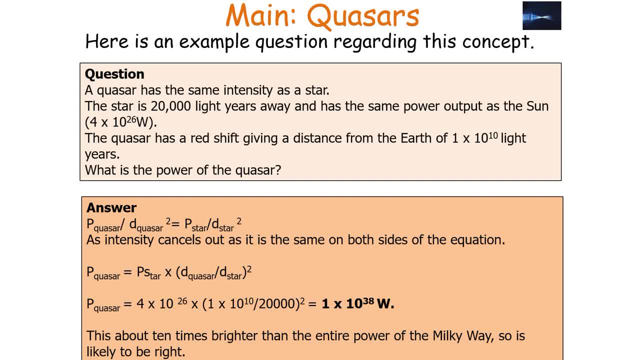 which is about 10 times brighter than the entire power of the Milky Way. So it's very, very likely to be right, because we know that a quasar is a super, super bright radio source, so it's likely to have a power a lot brighter than a. 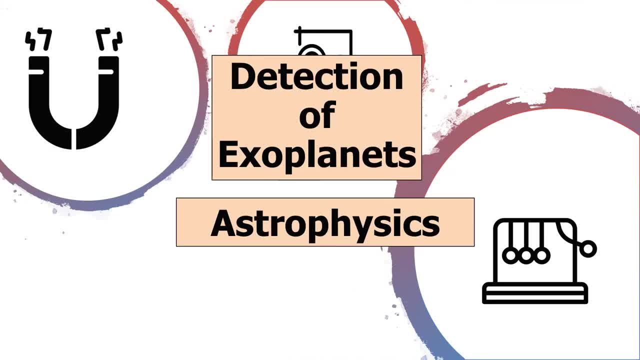 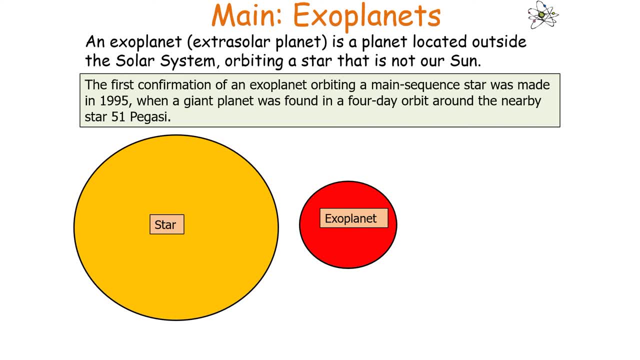 galaxy. Now the final topic we're going to look at in today's revision session is the detection of an exoplanet. Now, an exoplanet is a planet located outside the solar system, orbiting a star that is not our Sun. So the definition of an 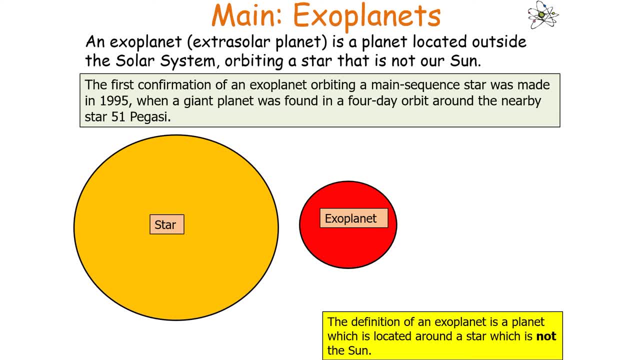 exoplanet is a planet which is located around a star which is not the Sun. Now, the first exoplanet we discovered orbiting a main sequence star was the Sunlight 51- Pegasi and a muscular spherical solar system called the Super Sun. And it's a planet which is located around a star which is not the Sun. Now, the first exoplanet we discovered orbiting a main sequence star was the Sunlight 51- Pegasi and a 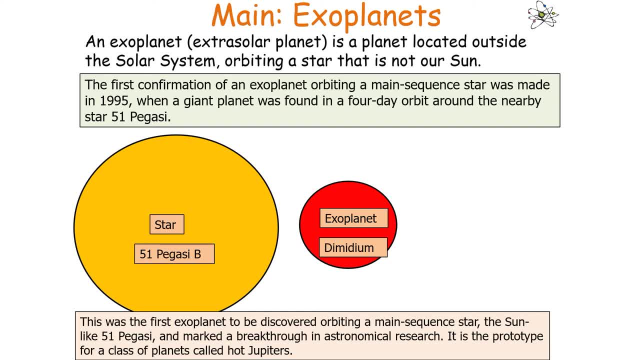 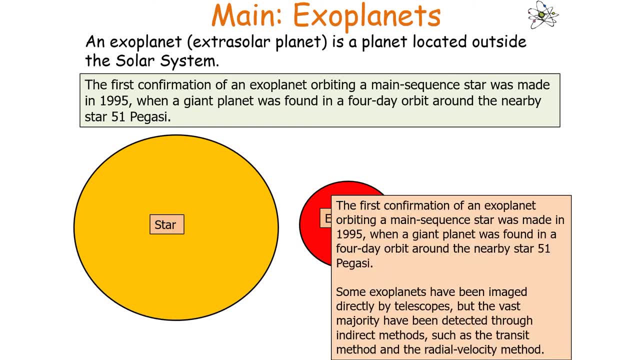 marked a breakthrough in astronomical research because they found a prototype for a class of planets called Hot Jupiters. Now some exoplanets have been imaged directly by telescopes, but the vast majority have been detected through indirect methods such as the transit method and the radial velocity. 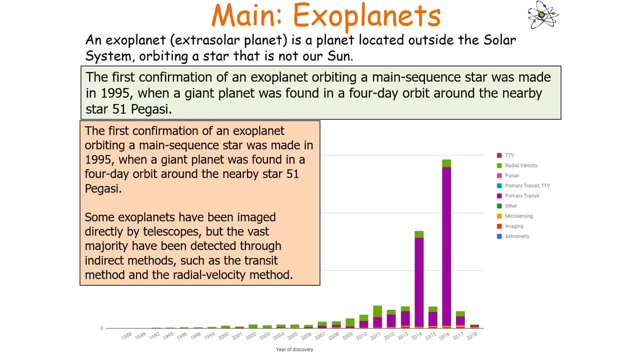 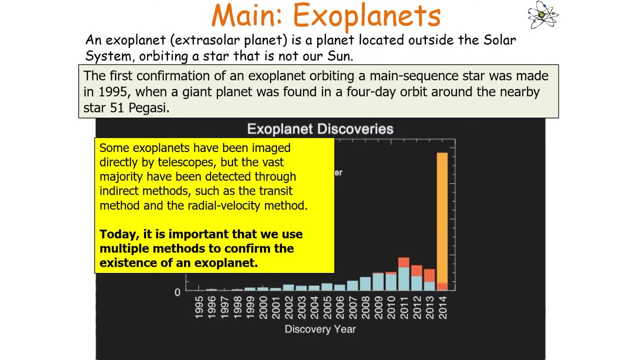 method. So, as you can see in the following image, there's a variety of different methods that were used to detect exoplanets in 2021.. Now, some exoplanets have been imaged directly, but the vast majority are used by indirect methods, so we've got to use multiple methods to confirm the existence of an exoplanet. 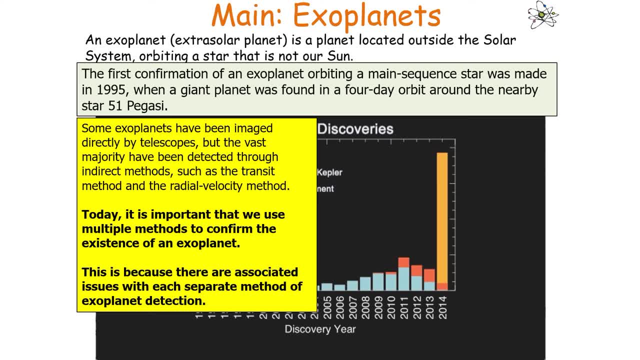 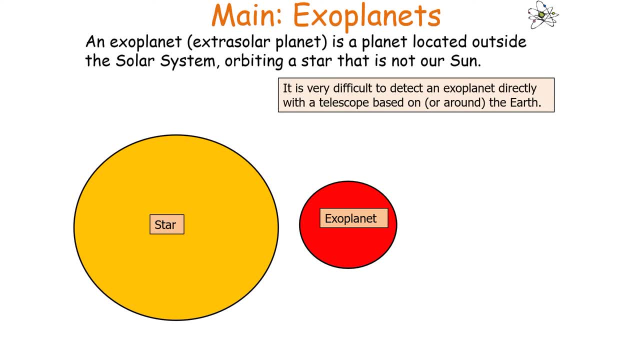 This is because there's an associated issue with each separate method of exoplanet detection. Now, if we just consider an exoplanet orbiting a star which is not our Sun, it's very difficult to detect an exoplanet directly with a telescope based on or around the Earth. 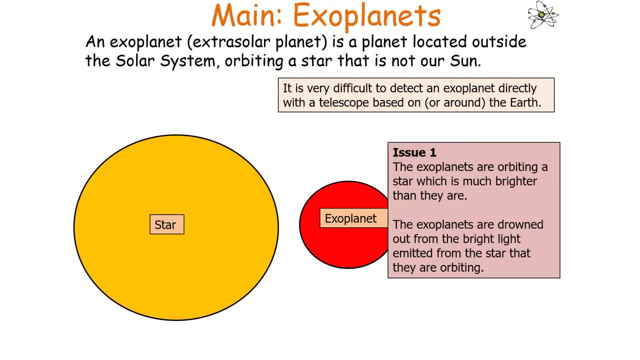 Because, firstly, the exoplanets are orbiting a star which is much brighter than they are. The exoplanets are drowned out by the bright light from the star which they are orbiting. The second issue is that the angular separation between the star and the exoplanet is much. 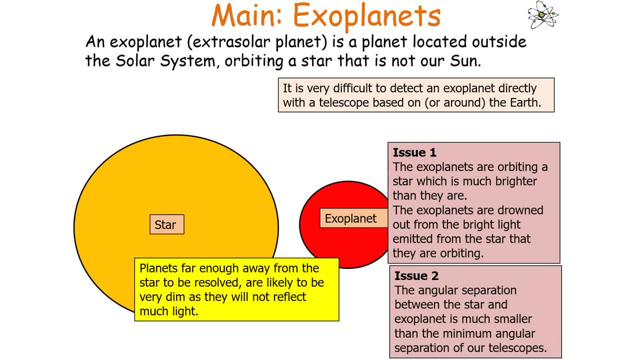 smaller than the minimum angular separation of our telescopes. Now, planets far enough away from a star to be resolved are likely to be very dim. because they're so far away from their star, they'll not reflect much light. Now, despite this issue, several exoplanets have been directly imaged. 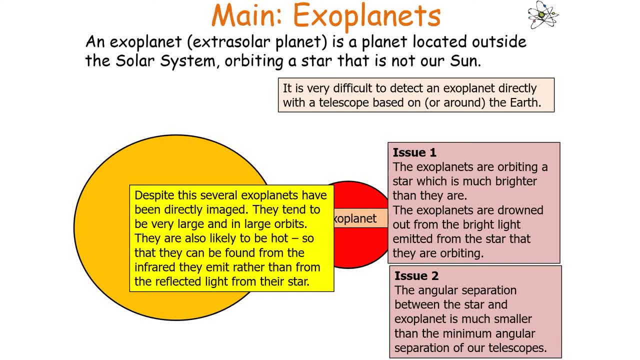 They tend to be very large and in very large orbits, and they also tend to be very hot, so they can be found from their infrared emission rather than the reflected light. Now it also helps if the planet orbits a brown dwarf or another dim star. Now technology has advanced and various masking techniques have been developed to block out. 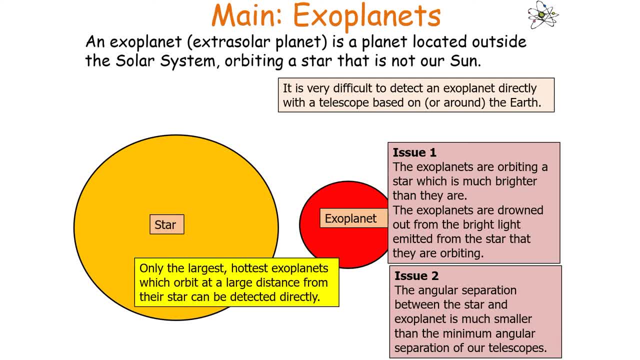 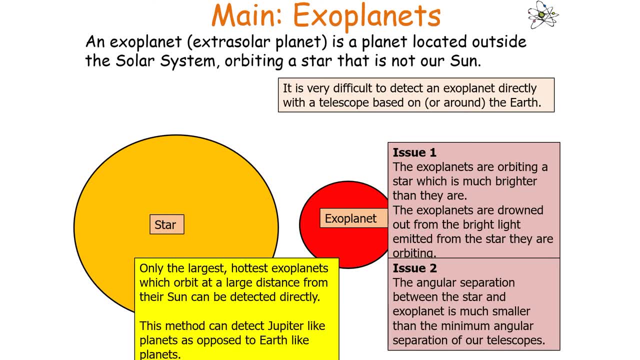 the light from stars so that planets orbiting may be directly imaged. But only the largest, hottest exoplanets which orbit at a large distance from their star can be detected directly. So this method can detect Jupiter-like planets as opposed to Earth-like planets. 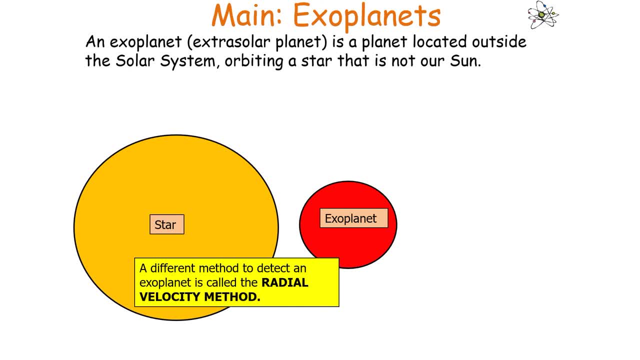 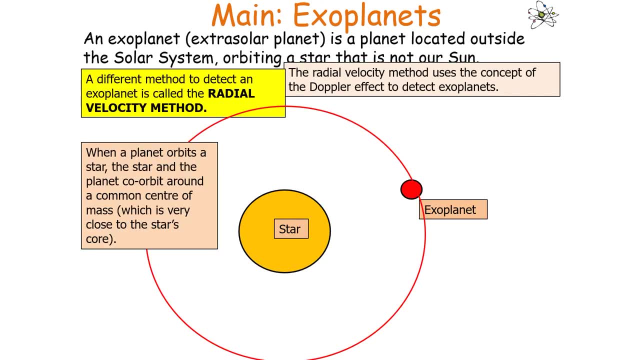 So other methods must be used to detect exoplanets. So a different method to detect exoplanets can be used to detect Jupiter-like planets. The first method to detect an exoplanet is called the radial velocity method. Now this uses the Doppler effect to detect exoplanets. 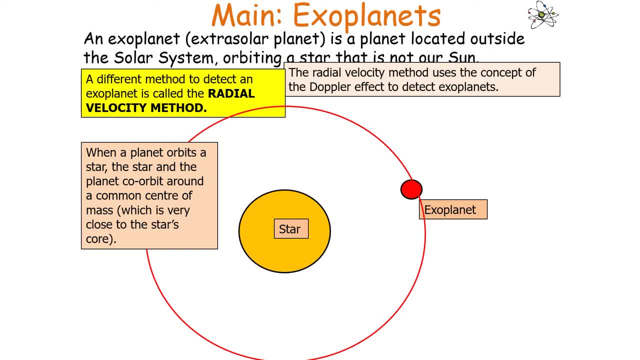 So when a planet orbits a star, the star and the planet co-orbit around a common centre of mass which is very close to the star's core. That's because most of the mass of the star system is found in the star. So this causes the star to have a slight variation and wobble on its axis, whilst the exoplanet 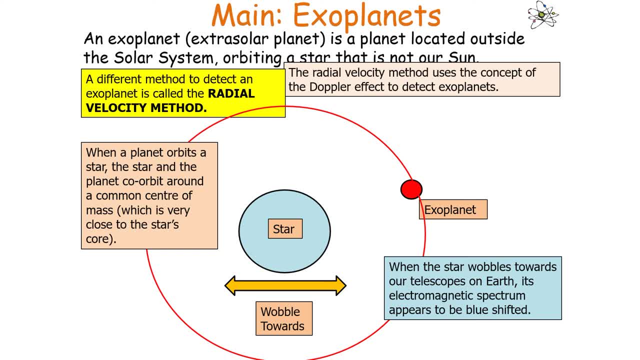 orbits the star. So as the star wobbles towards our telescopes on Earth, the electromagnetic spectrum it emits appears to be blue shifted, Whilst as the star wobbles away from our telescope on Earth, its electromagnetic radiation it emits appears to be red shifted. 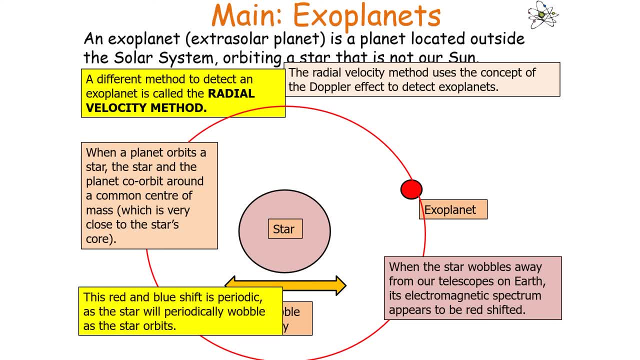 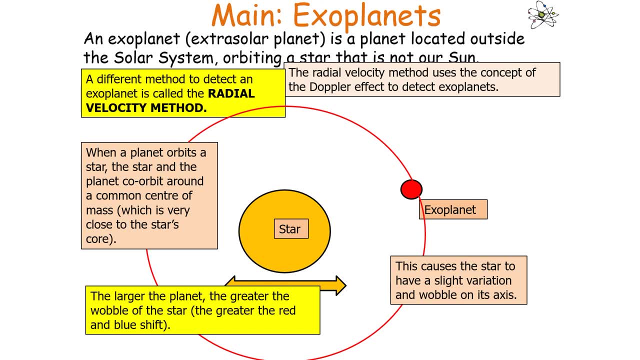 Now this red shift and blue shift is periodic, as the star will periodically wobble as the star orbits. So we can work things out with the Doppler spectroscopy. Now, the larger the planet, the greater the wobble of the star. So the greater the red shift and blue shift, The smaller the planet, the less the wobble. 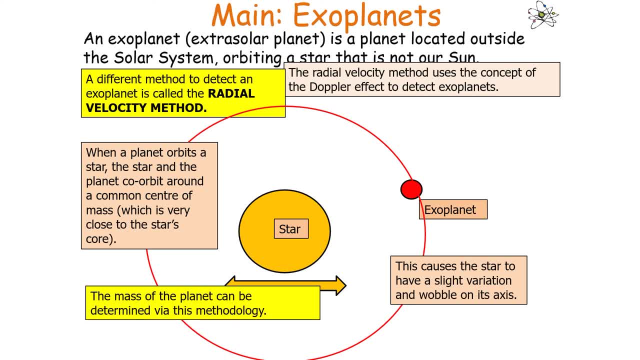 of the star And the less the red and blue shift. So the mass of the planet can be determined via this methodology. Now, for example, we can see a magnificent red shift, So the mass of the planet can be determined via this methodology. 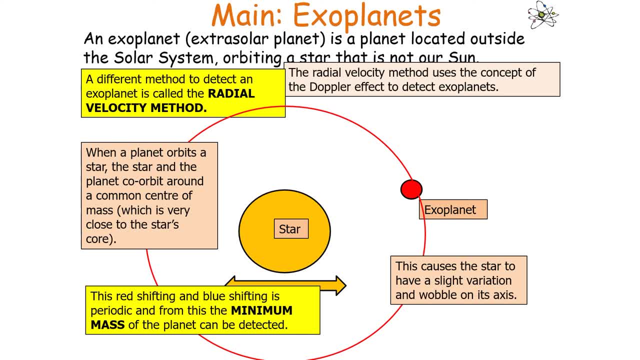 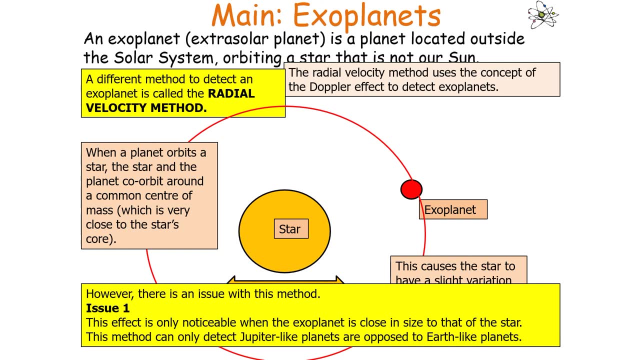 Red shifting and blue shifting is periodic, and from this the minimum mass of the planet can be detected. however, there are issues with this method. This effect is only noticeable when the exoplanet is close in size to that of the star, so this method can only detect Jupiter-like planets, as opposed to Earth-like planets. 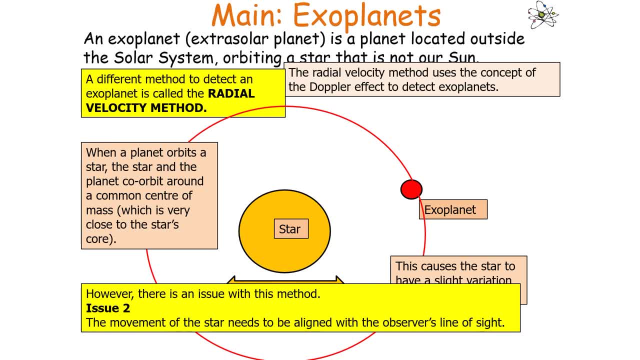 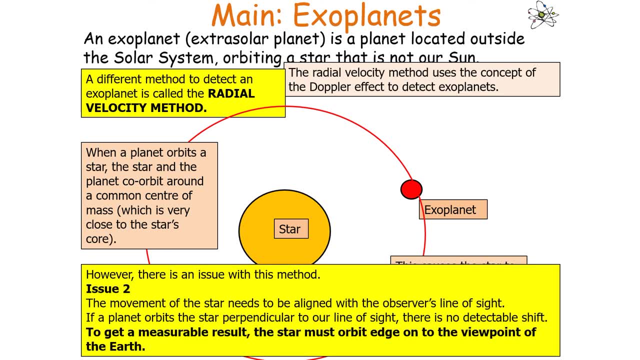 The second issue is that the movement of the star needs to be aligned with the observer's line of sight. If a planet orbits the star perpendicular to our line of sight, there is no detectable shift. As a measurable result, the star must orbit edge on to the viewpoint of the Earth. 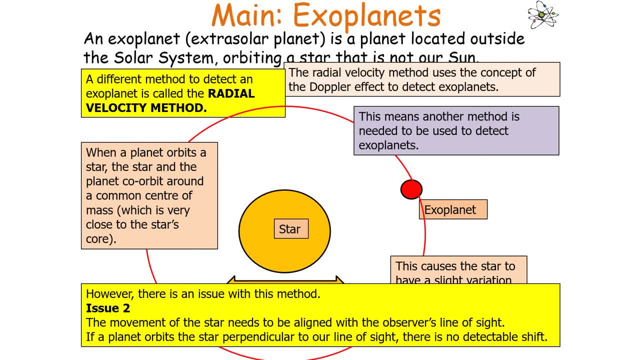 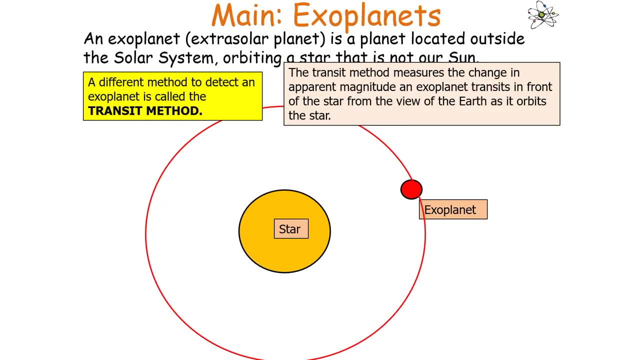 So this means that if a planet orbits the star perpendicular to our line of sight, there is no detectable shift. This means another method is needed to detect exoplanets, So a different method is used, which is called the transit method. The transit method measures the change in apparent magnitude an exoplanet transits in. 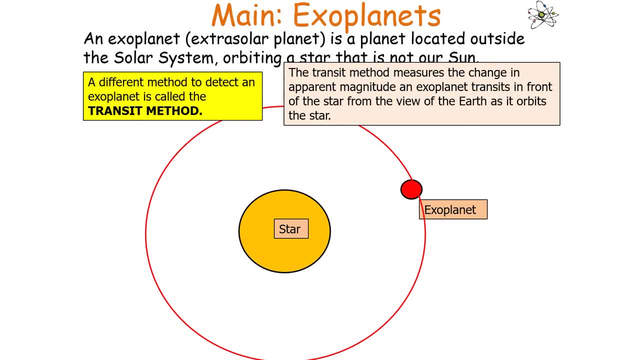 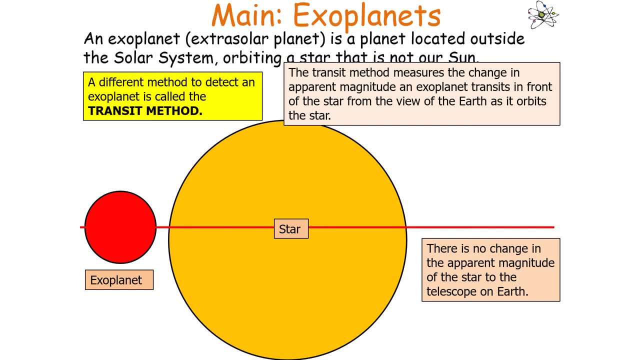 front of the star from the view of the Earth as it orbits the star. So as the exoplanet moves across the planet, It will show that there appears to be a dimming in the output of the star. So at this point there is no change in the apparent magnitude of the star to the telescope. 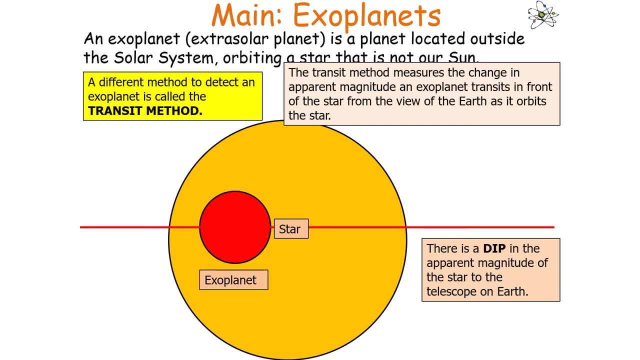 on Earth. Here, as the exoplanet passes in front of the star, there is a dip in the apparent magnitude of the star to the telescope on Earth. So the larger the exoplanet compared to the star, the greater the dip in apparent magnitude. 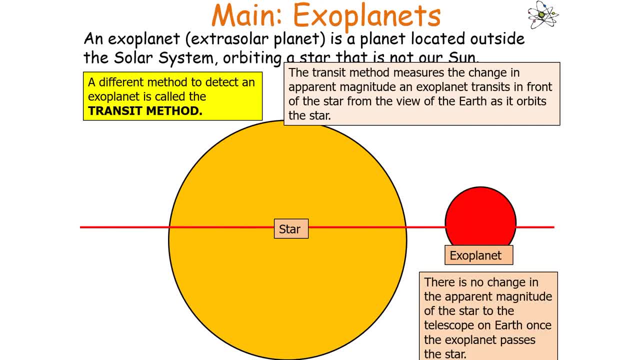 The further away the exoplanet from the star, the longer the dip in apparent magnitude. And once the star passes across the star, There is then no change in the apparent magnitude. The apparent magnitude returns to its original value. So you can look at the light curves of stars. 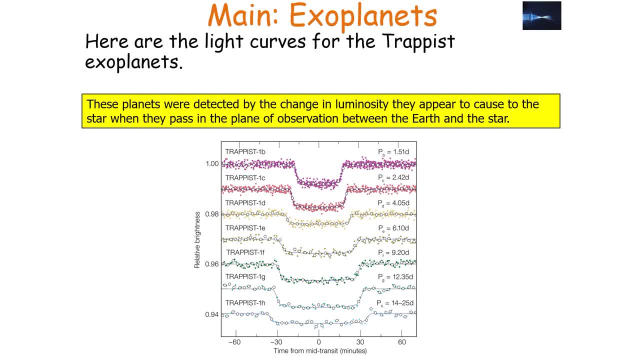 So this star has several planets orbiting around it and they were detected by the change in luminosity they appear to cause to the star when they pass in the plane of observation between the Earth and the star. So the bigger a planet, the larger the drop in apparent magnitude. 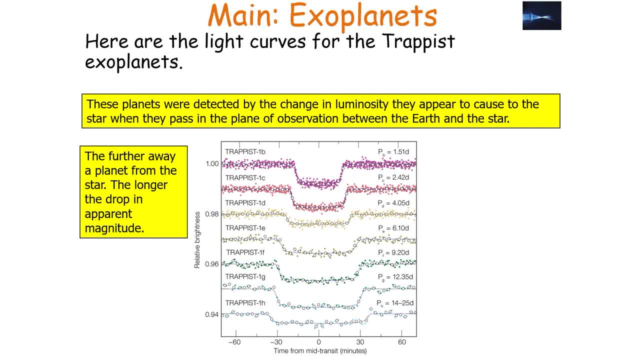 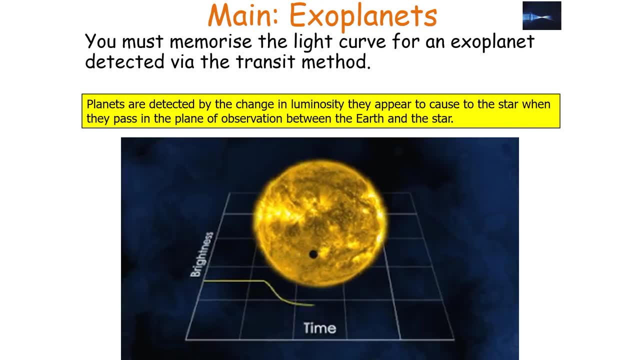 And the further away a planet from the star, the longer the drop in apparent magnitude. So this method allows you to determine the radius of a planet, the radius of the Earth and the radius of the exoplanet of a planet and its orbital distance from the star. so you can observe this with the following images. 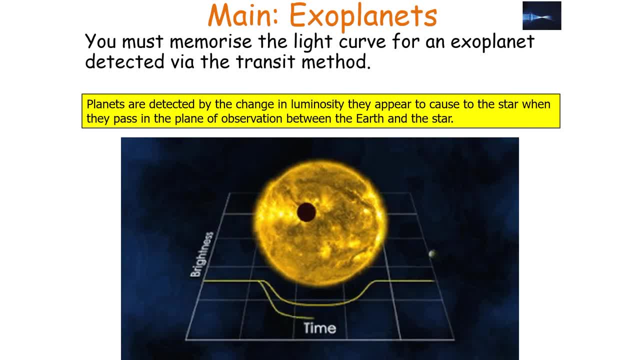 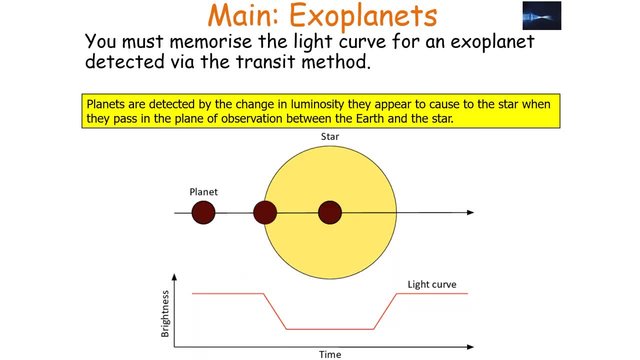 shown here. so you can see that as the star moves across, so as the planet moves across the star, you observe a dip in brightness in the output of the star. and again you can see here that as the star moves, as the plan moves across the star, you will have this dip in the light curve. now it's important. 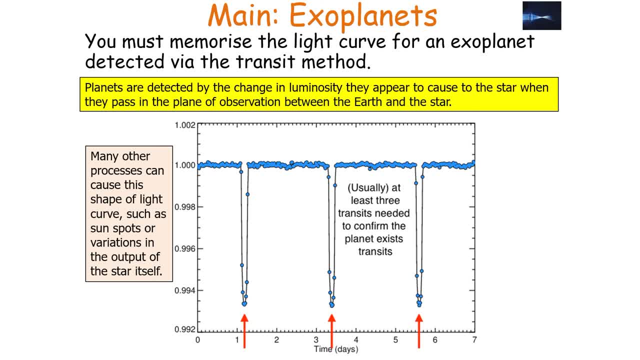 to also note that many other processes can cause this shape of light curve, such as a sunspot or a variation in the output of the star itself and other stellar objects can cause this dip in apparent magnitude, but the the existence of an exoplanet is confirmed if these dips in the light curve are. 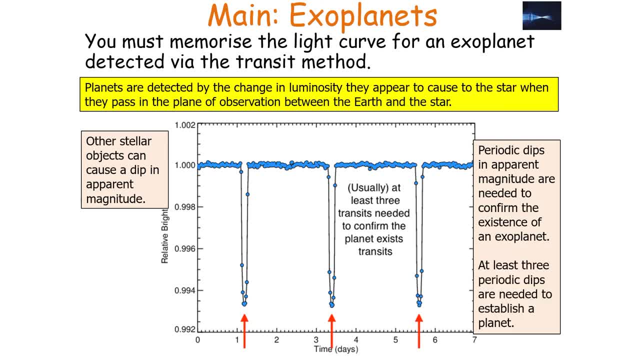 periodic. now at least three periodic dips are needed to establish a planet, so this can lead to various issues. so number one: one issue in the transit method is that a dip in light curve can be caused by other effects. issue two is that periodic dips can take a very long time to. 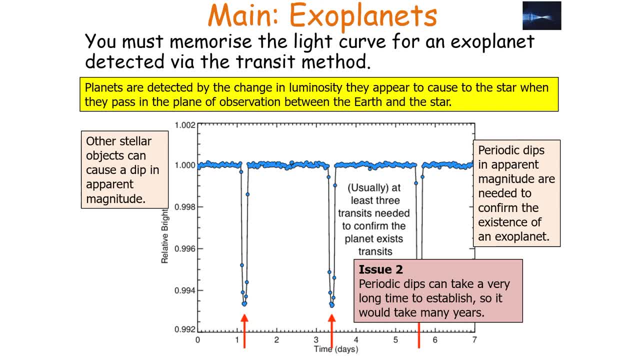 establish, so it could take many years to complete. so this is a very important issue in the transit method. and number three is that alignment must be correct for planets and stars to eclipse in the plane of the earth, which is quite unlikely. so even if it is aligned, the transit is likely to only last a tiny fraction of the whole orbital. 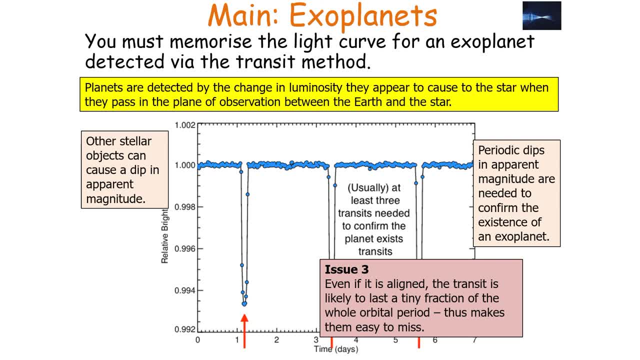 period, so it makes it very easy to miss if you're not studying the star closely. so this alignment issue means that this method can only be used to confirm existing exoplanets, so if no dip is observed, it doesn't not always mean that there's no planet.